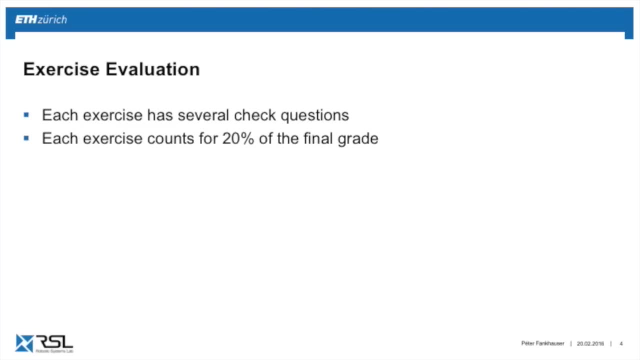 And that those are the ones we're going to go through when we grade. We have five exercises in. each of them count 20 percent. We encourage teamwork, but all of you have to show their results either on their personal laptop or on one of the PCs in the back to us individually. 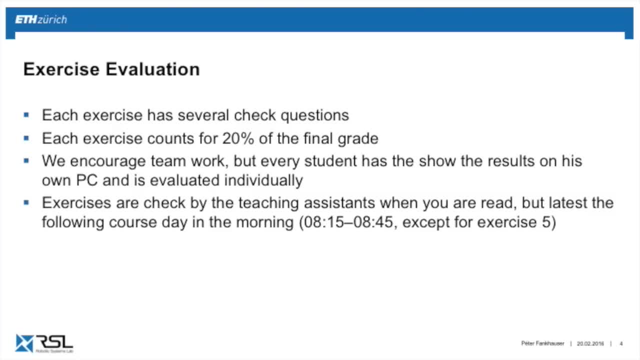 Like I said, exercises are checked by teaching assistants or, the latest, the following course in the morning, which means in the morning 815 to 845, that's the time where you can come by and show us the exercise. come early such that we can start in the lecture on time. 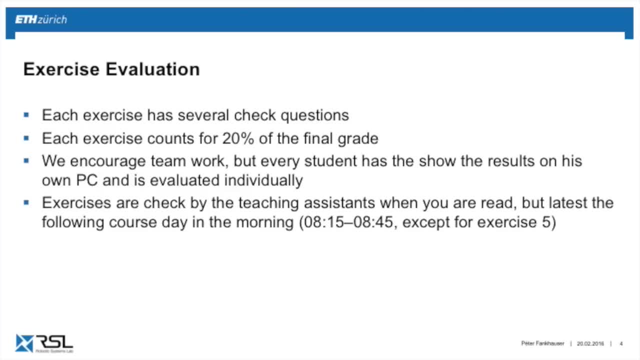 This is except for exercise five, where you have to show it at the very end of the course because that's a shorter one And that's where the course will finish. Let us know once you're done, so we can check you gradually, so not everybody comes in five minutes before the lecture starts. 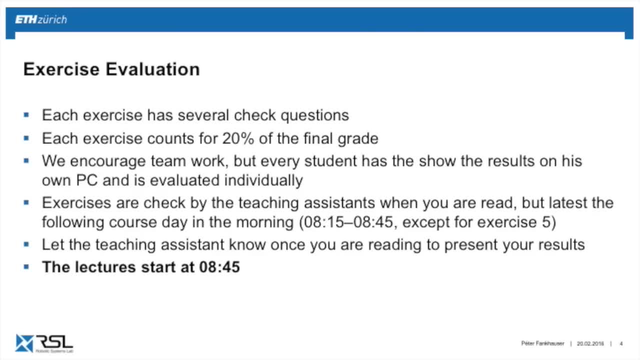 And important for those who have already given us, shown us the exercise, the lecture, the theoretical part will start 845.. So you can show 815 to 845, and then, for those who have shown it, come here at 845. 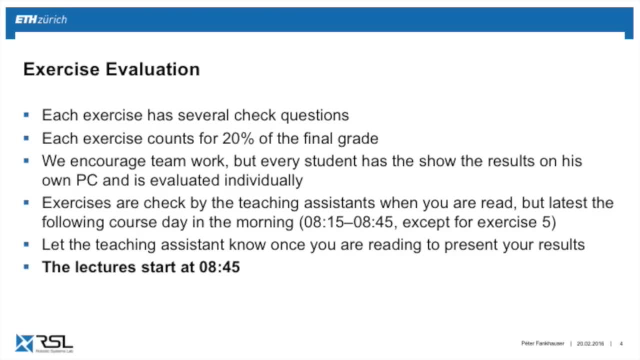 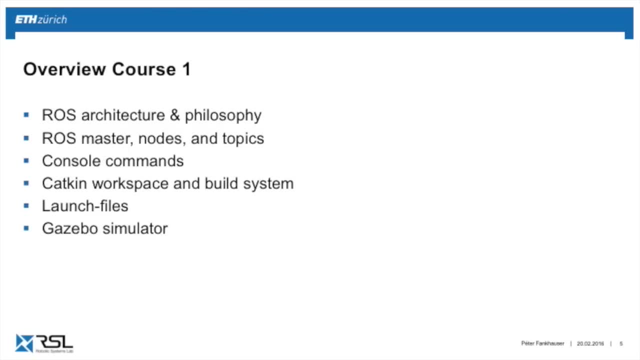 But the best is if you show it during the morning, especially for the easy ones. Just raise your hand and then we can check on you and then you can actually leave, Okay, So in course one we'll talk about the ROS philosophy, the architecture and go through the important concepts like the ROS master, ROS nodes and topics. 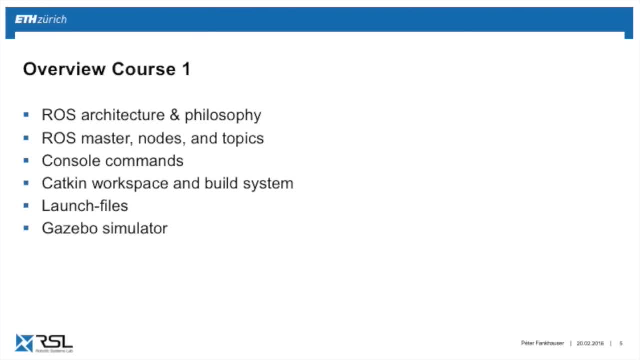 You'll learn how to use your console to do basic commands and analysis of what's running on your PC, And we talk about how you build your nodes in your system with the Katkin workspace. And then in the exercise you're going to be using launch files and the Gazebo simulation. 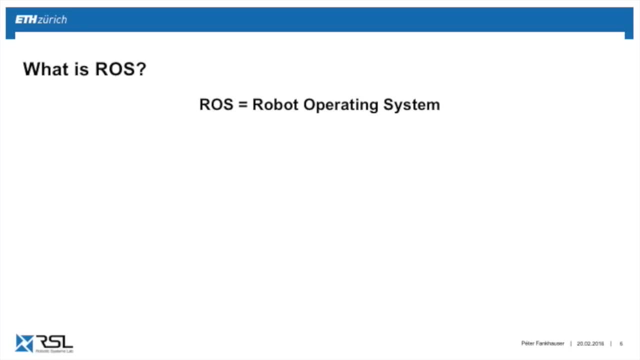 So what is ROS? ROS stands for the Robot Operating System. It's not actually an operating system like the ones you have installed at Windows, Mac or Ubuntu. It's more a middleware that lives between the actual operating system and the program that you write. 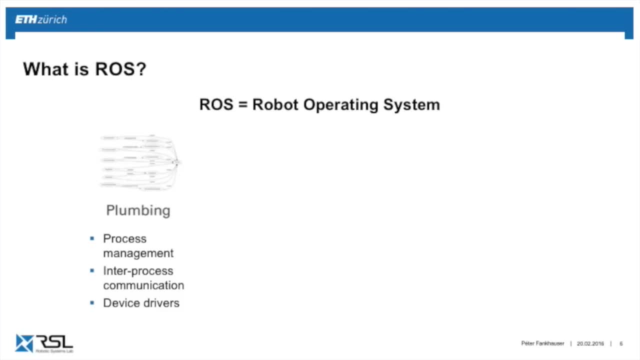 It has four different elements. One is the plumbing, which means that you have multiple programs running, And ROS is a very complex program. It's a very complex program And ROS enables you, these programs, to communicate between each other. Also, it provides a bunch of device drivers that allow you to easily communicate with your hardware. 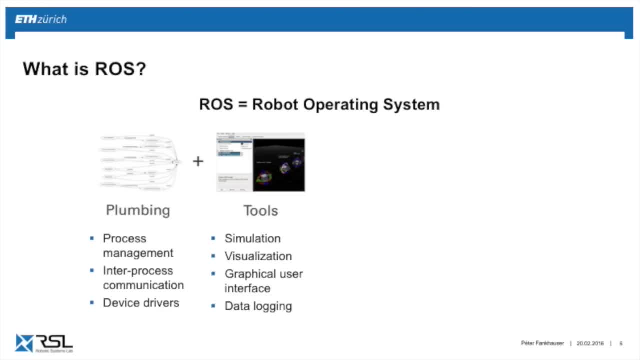 A second part is that there's many basic tools which are important when you work with robots, being it simulations, visualizations, a graphical user interface that you can adapt or basic tools like data logging. So all these tools were written once and you can reuse them to facilitate your work when you work with robots. 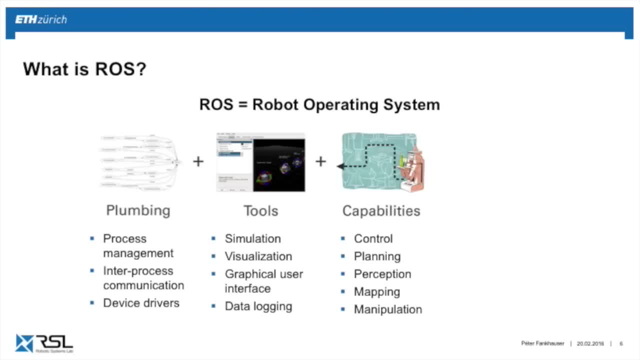 There's a bunch of capabilities in ROS, being it for control, planning, perception, mapping, etc. Many people provide to this ecosystem of ROS so you can make use of existing tools. So if you're an expert in planning, you don't have to write your mapping algorithms yourself. 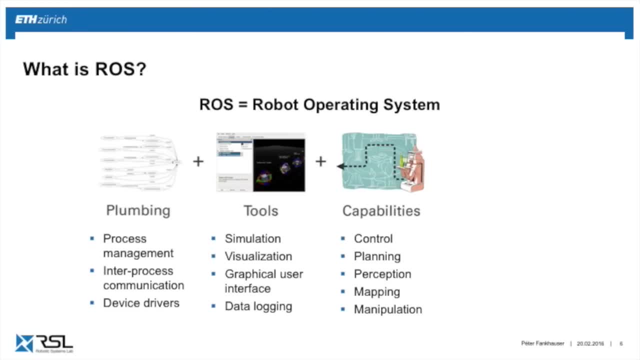 You take some of the shelf and develop your own in your specific area of expertise. Lastly, ROS is a big ecosystem. The software is organized in packages Such as you can easily install and use them, And ROS provides entire software distribution. And there's many, many tutorials, and you're going to work with some of those online available in documentation. 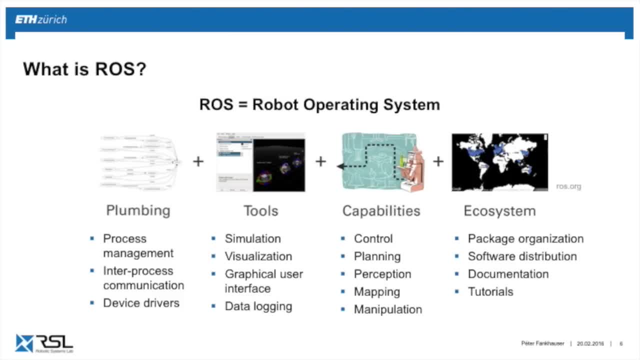 For this course, we'll mainly work with the plumbing, the tools and the ecosystem, The capabilities. those are the things you're going to dive more deeply in during the semester work or other work where you go towards the algorithms. We provide you here the basics for ROS, which are the tools. 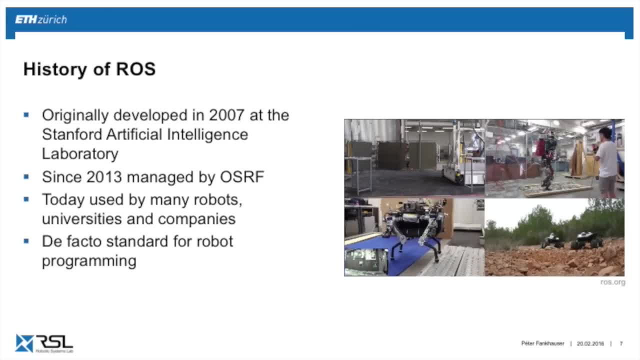 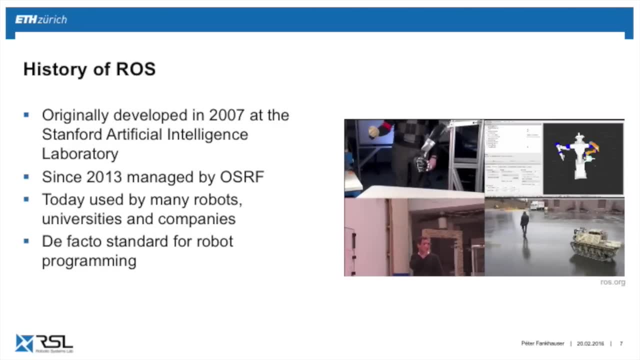 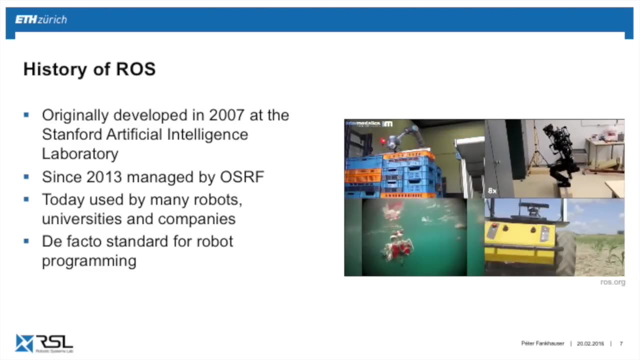 The inter-process communications. A little bit to the history of ROS: It was developed in 2007 at the Stanford Artificial Intelligence Laboratory and then was managed by Willow Garage, which was taken over, and then, since 2013,, it's now managed by the Open Source Robotics Foundation. 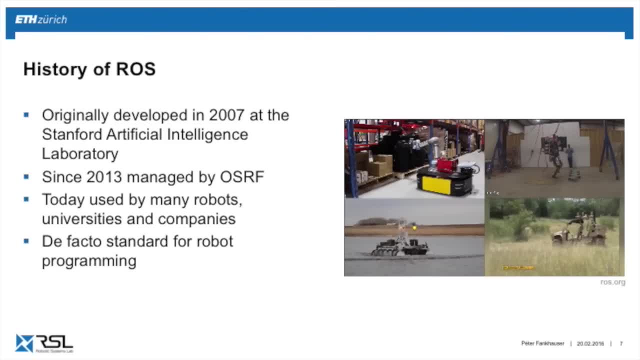 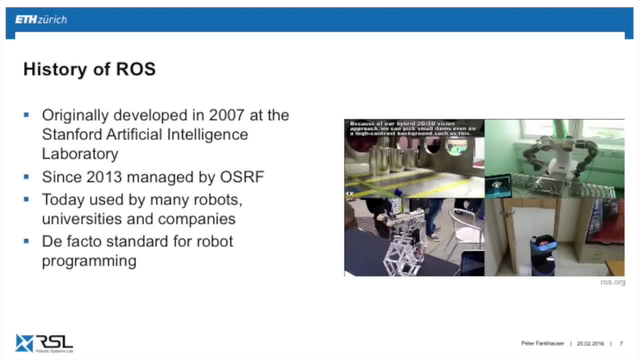 Today, ROS is used by many, many robots, and you see some of them in the videos. These range from universities to companies who use this industry. These range from universities to companies who use this industry. These range from universities to companies who use this industry. 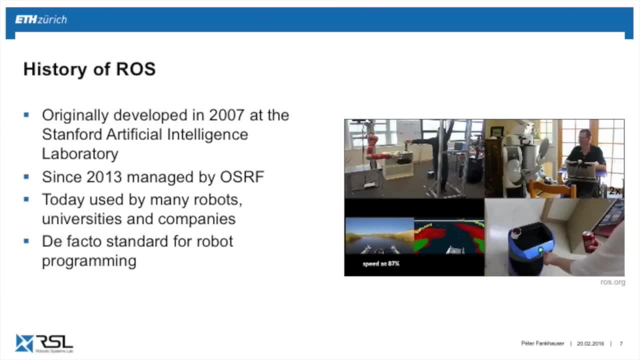 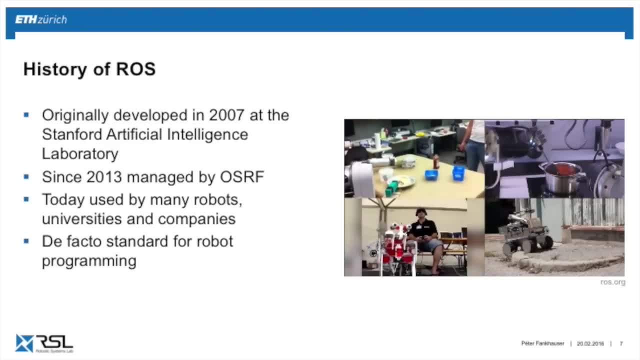 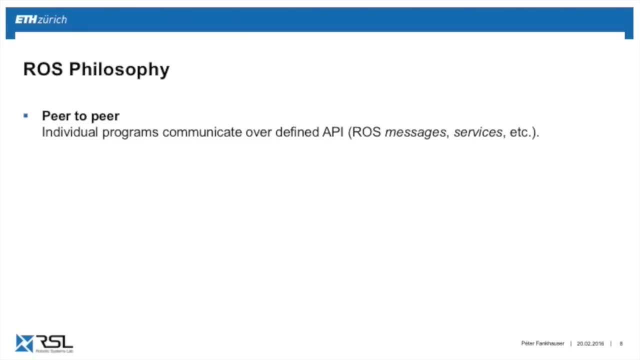 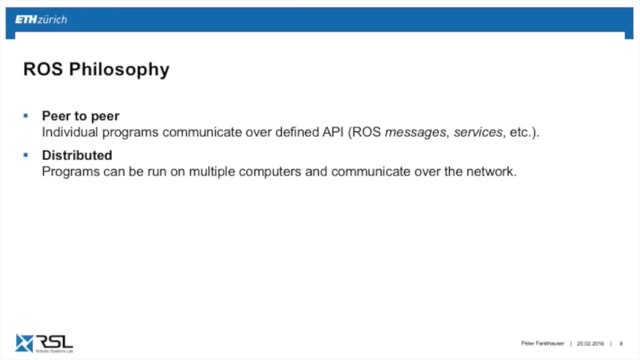 running on your system. Now, since it's peer-to-peer, it can be distributed on multiple PCs. so if you have a robot which has a computer in your computer, it communicates over wireless and it doesn't matter on which nodes, on which PCs the nodes run, since the APIs and the communication runs also not only. 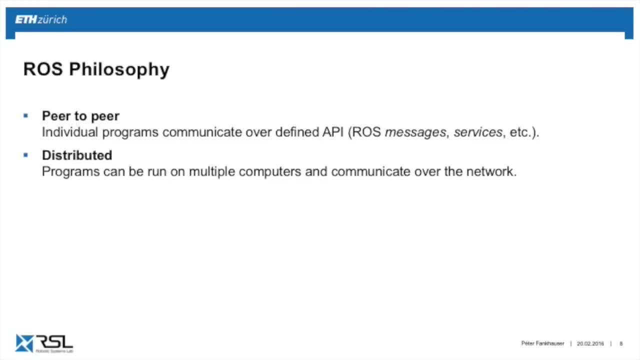 on your PC, but also over wireless. You can build a big distributed system with multiple PCs easily with ROS. It's multilingual means: you can use any of these existing languages, which provides a ROS client library. We'll mainly work with C++ in this course, but, such as you know, there exists the libraries. 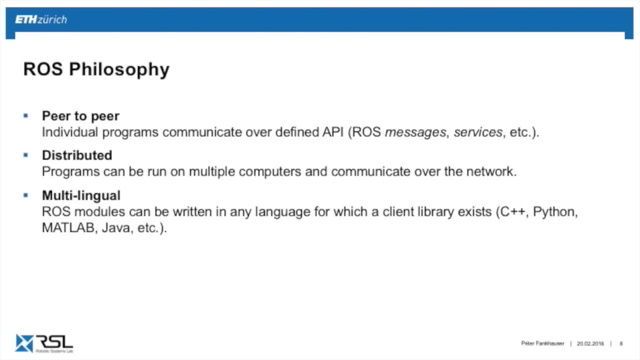 for Python, MATLAB and Java, and these can be mixed and matched. It's lightweight in the sense that ROS is not It provides all the algorithms. The idea is that you take existing standalone libraries and wrap them with the ROS layer, such that you enable existing algorithms to communicate and work with other tools together. 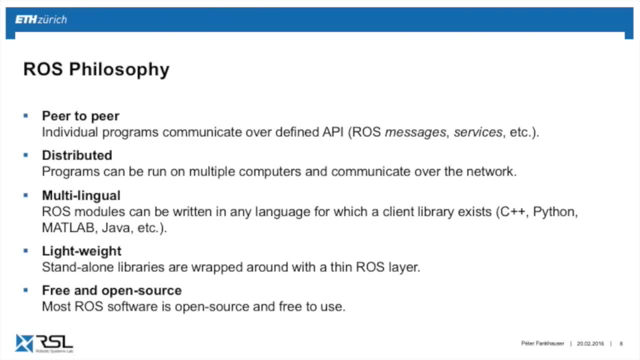 on your robot. And finally, ROS is great because it's free and open source, so, to the very core, you can dive in and check for things and if you find a bug you can do an issue or actually fix it yourself and do extensions of ROS. 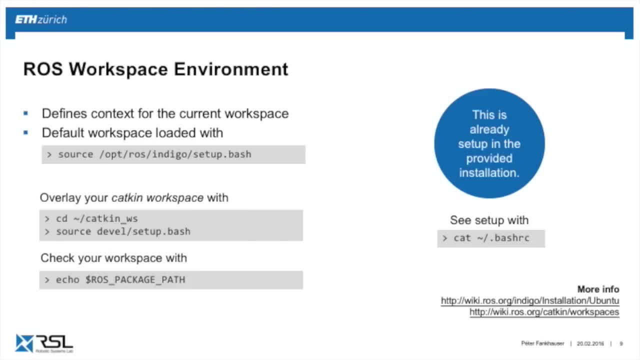 So what's the next step? What's the next step? What's the next step? So one important element that you'll see is the ROS workspace environment. This defines actually the context on where you're working in the ROS environment. There's a standard when you install it in the environment, which is under if you type. 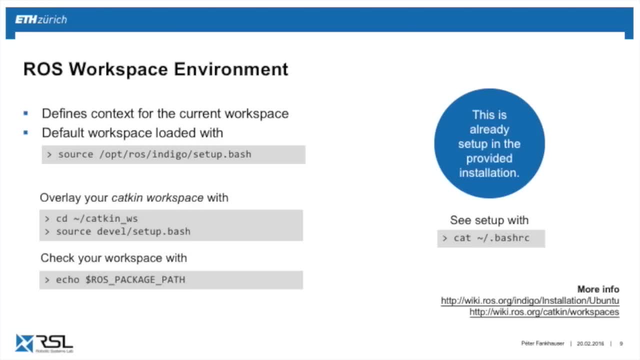 in this command which loads the ROS version and then the environment that you need And, importantly, you can overlay these environments. So in your PC we already pre-installed one which we set up in the standard folder, the catkin-workspacecom. 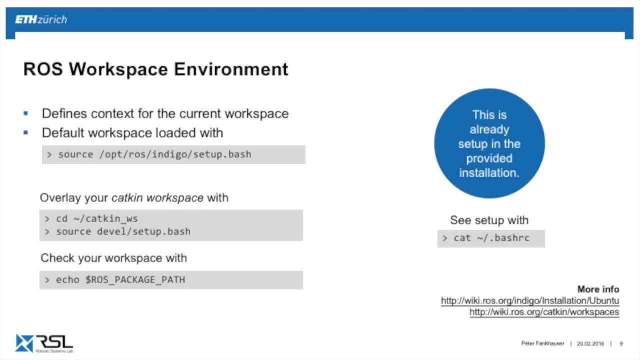 And by default, whenever you open a console, we load on your virtual machine that we provided you the standard workspace of your catkin environment with this command. You can check the environment with this command and you can also see how we set up your PC. 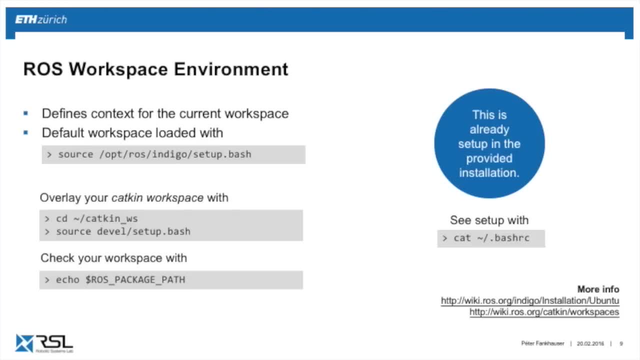 with this command in the future if you want to install your own PC, So this is already set up. This is only for future reference. Now, one important element that you'll see is that you can set up your own virtual machine, So this is already set up. 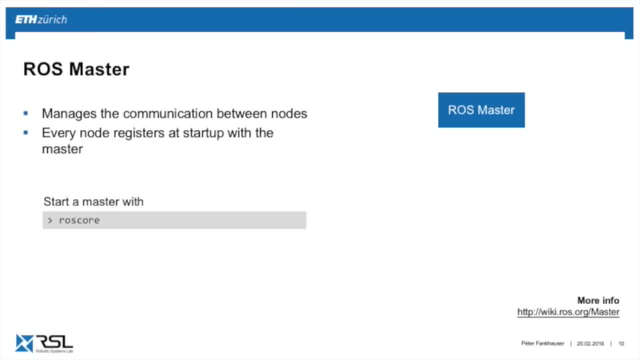 This is only for future reference. And the most important element is the ROS master. This manages the communication between your nodes, So at startup, when a node comes up, it needs to register with your master And the master makes sure that all the nodes can communicate with each other. 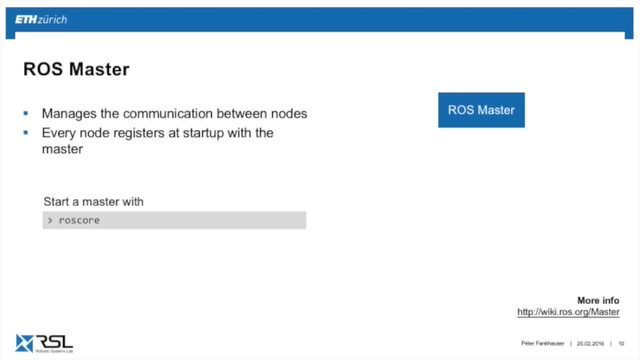 You can start in the console with ROS master, which is simply typing in ROS core. ROS core has multiple elements, one of which is the ROS master. It ROS knows power. Yes. Next action: Okay is essentially a program that runs on your PC. 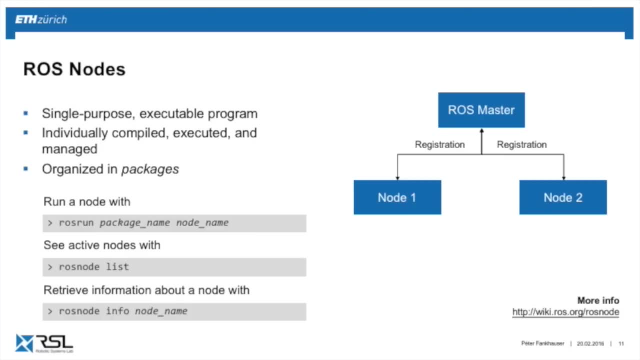 So it's a single purpose executable program. You can compile them individually, run them and manage them individually. So those are the building blocks of your program. These nodes are organized in packages, So whenever we mean a package name, it's essentially the name of the package. 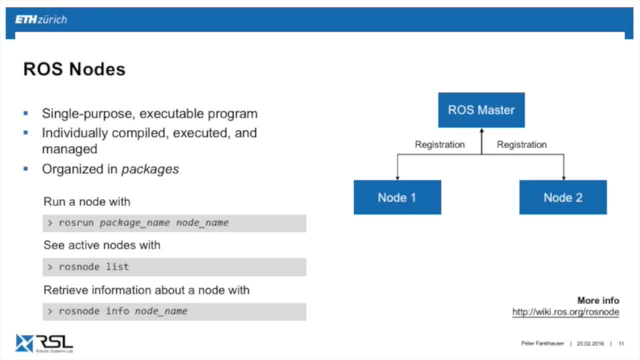 And then in there you can have multiple nodes. You see how here in the example ROS master, each individual node needs to register with the master such that it enables the communication To run a node, and you'll use this during the exercise. 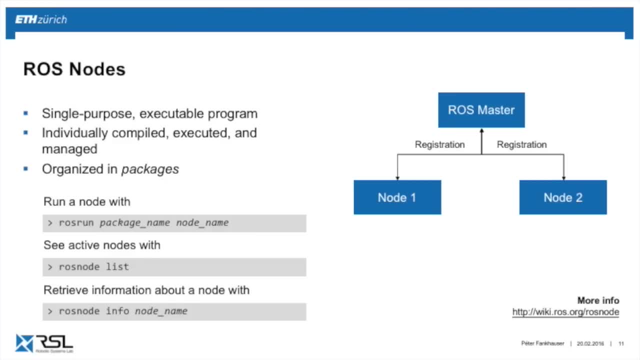 you type in ROS run, then the package name and then the name of your executable. Once you've done that, you can look at the list of all the program that runs by typing in ROS node list, which lists you all the active ROS nodes. 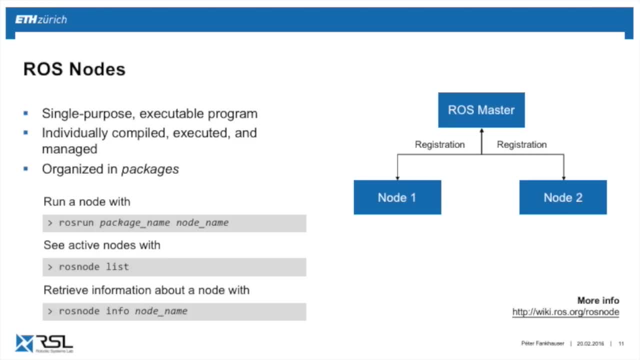 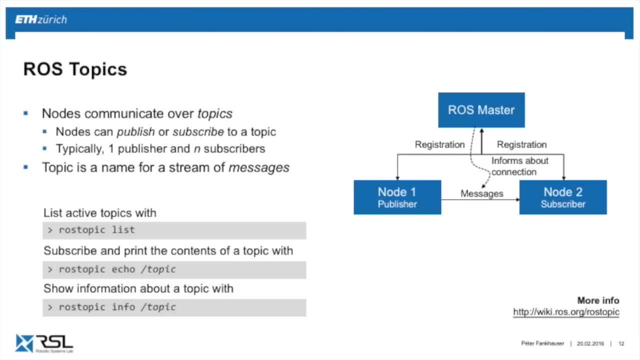 And then, if you need further information, specific information about one of the ROS nodes, you type in ROS node info and then the name of the node, And then it spits out all the information about the node. How do nodes communicate with each other? 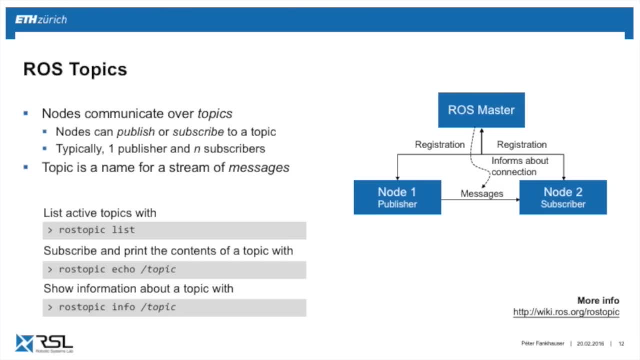 They do it through ROS topics. So one node can publish and subscribe to a topic And essentially a topic is a stream of messaging messages that are transferred between the nodes. so in this example, once the nodes one and two have registered with ross master the node, one can tell: okay, i'm a publisher on these, this topic. 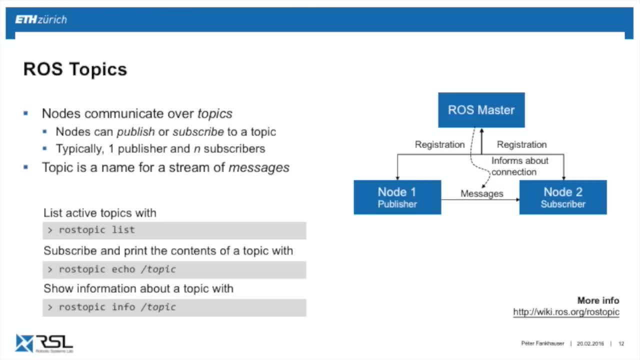 and ross. node two can subscribe to this topic, so the message flows from the publisher to the subscriber. enter us, master. make sure to inform about this connection here. so the publisher publishes on a topic name, which is the name um, under which these messages are published, and then you can have not only one but multiple nodes that subscribe to this. 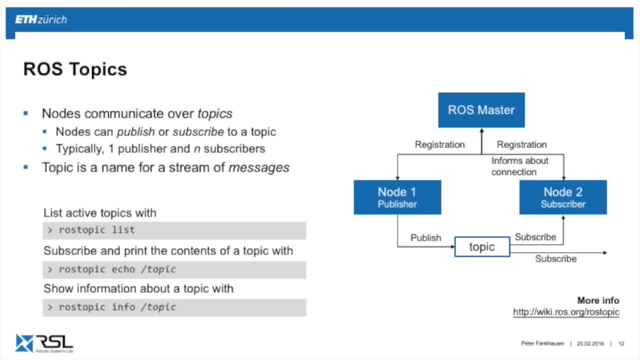 information, but typically it flows from one known to n other nodes. to look at the list that you have by provided by the nodes that run on your system, you can type in ross topic list if your list or your list of the nodes that are running on your system. you can type in ros topic list if your list or 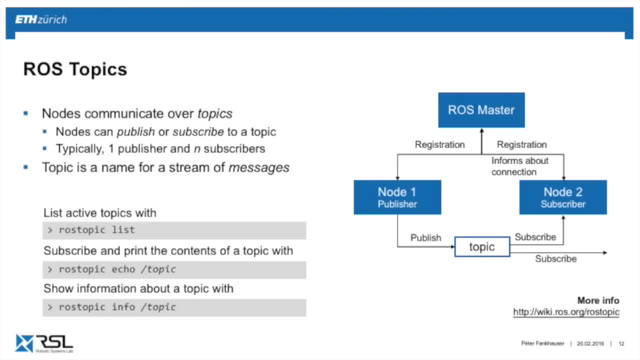 of all the topics You can already in a console. you can subscribe to a topic by typing in ROS topic echo, So it's printing out information and then the topic name. This will subscribe to this topic and show you the contents on the console. 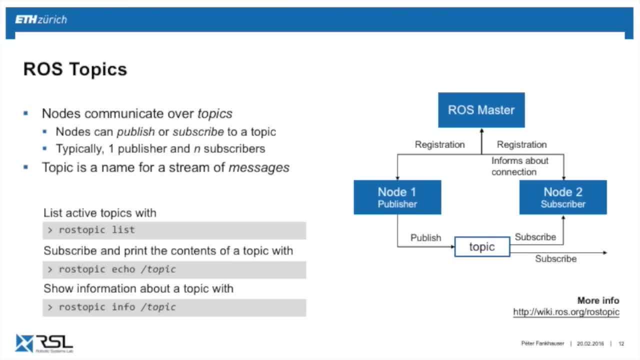 And if you need information about a topic, again like with the notes, you type in ROS topic info and then the topic name I always provide here links to the documentation of ROS. So if you need further information, just you can download PDF from our website. 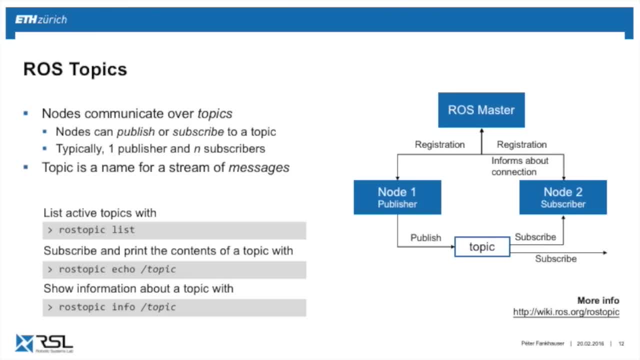 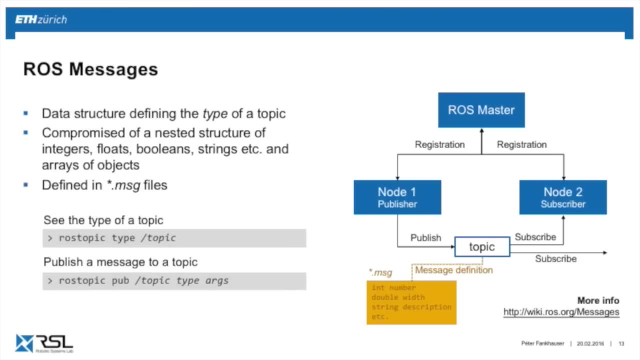 from the slides, type it in or click on it, And so you get much, much more in-depth information on these specific topics. Now, on these ROS topics, the notes publish messages. So essentially, the message defines the data structure of the information that flows from one note to the others. 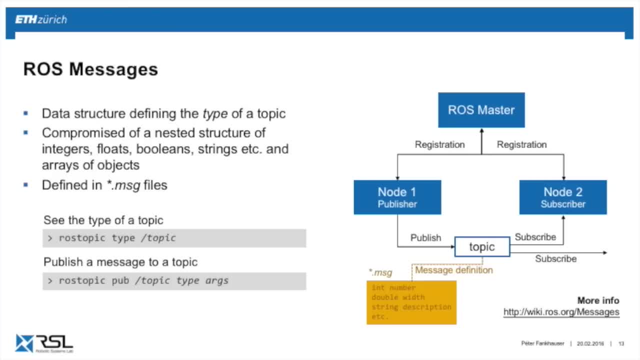 It's essentially a compromised of simple types such as integers, floats, Booleans, strings, et cetera, and also arrays of these objects, And they can be nested, So one message can be included in the other one, And we'll see an example in a second. 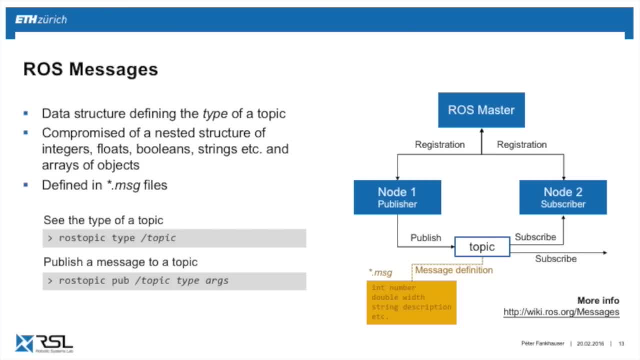 If you have a topic, you need to know the type of it. You can type in ROS, topic type and then the node name, the topic name, sorry- And if you need to publish on the topic, so if there's a subscriber but you have, you don't have the. 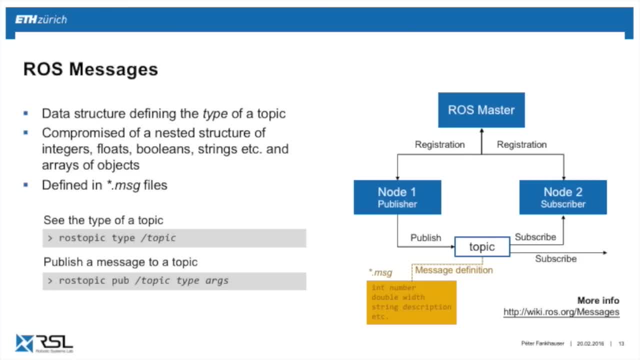 node, yet that publishes it. you can publish from the console the tool with ROS topic publishing, then the topic name, then you type in the type And then, if you click tab- tab is a very important command- It auto completes the rest of the structure. 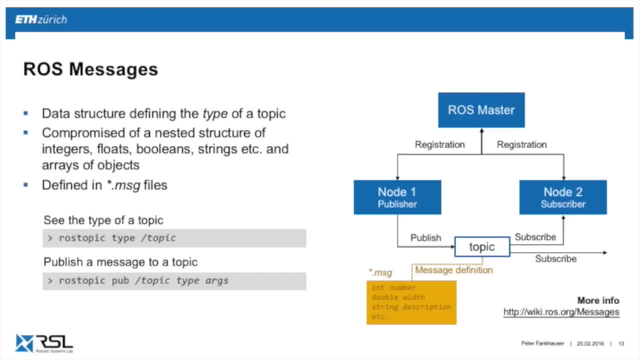 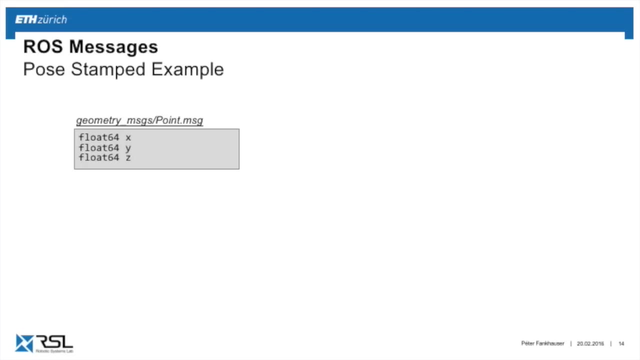 such as you can replace the arguments very easily and then publish on this topic from your console. So in this example we have a publisher publishes on the topic And the topic is inherently coupled with a message definition. Here's an example of a message definition. 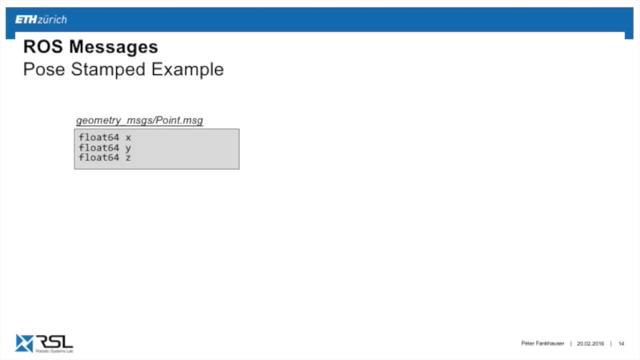 which in this case come from the package geometry messages and is of the type point message. So this is essentially a text file with the ending dot MSG message, And within this file you can easily read the contents of it yourself and write your own messages. 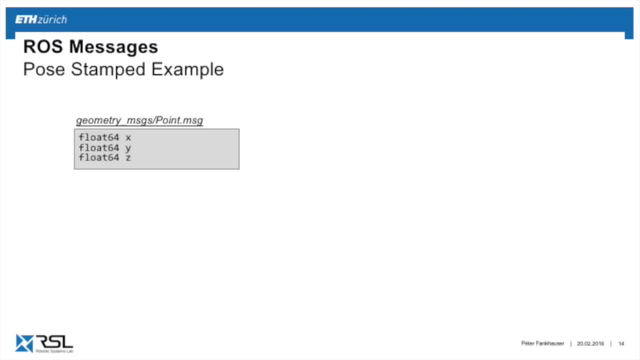 So in this case we have four floats, four floats, 64 doubles with the coordinates X, Y and Z. Here's another example, more complicated, from the sensor messages topic. This is an image, So on the top you'll have a header. 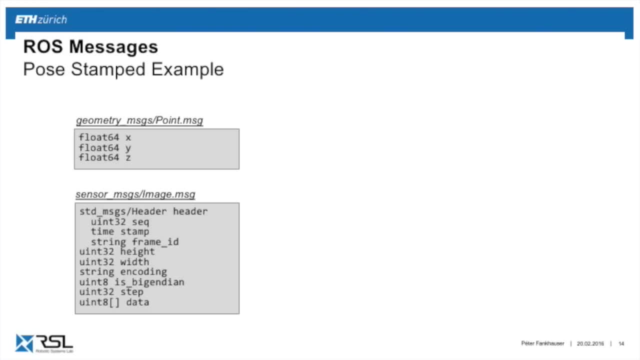 which means there's a sequence number, a timestamp and the frame ID. Sometimes this is important if you have geometrical information to associate it with a frame, And then you have height, width of an image and then information about encoding, So you can see the data of the image. 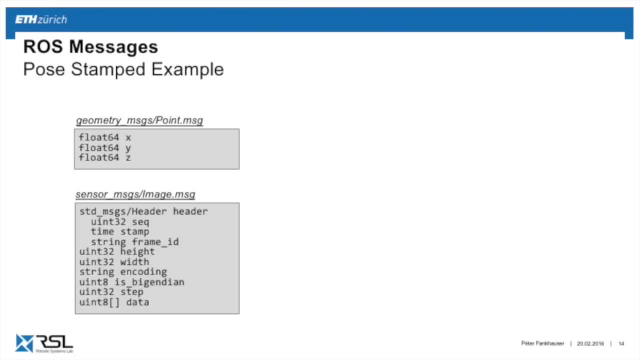 and then, as an array, the data of the image itself. Of course you can print this in the console, but it's not gonna show as an image. There's other tools for that that we learn later. In this example, again, we have a header. 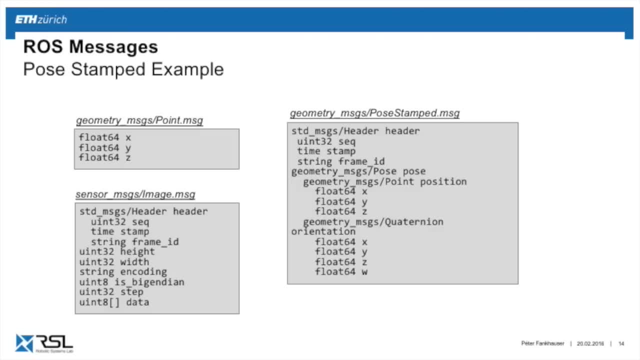 So this is a pose message. A pose is a compromise of a position and orientation, And here we say: okay, the pose, you have a position: X, Y, Z, and the rotation is here given as a quaternion with four numbers. 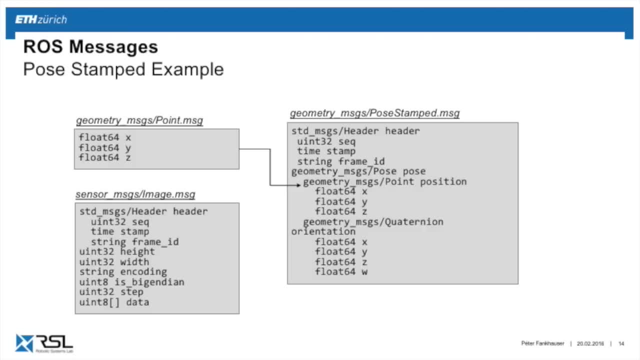 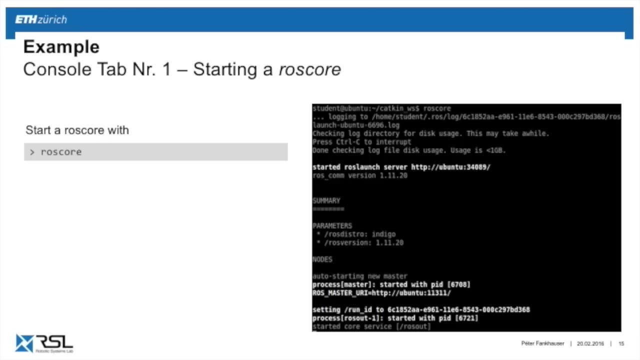 And, as you can see, this message is compromised- of another message type. So the point defines here the position. So these messages can be nested into each other, making it very easy to create new ones and building up on other standards. Now for the people who are running already. 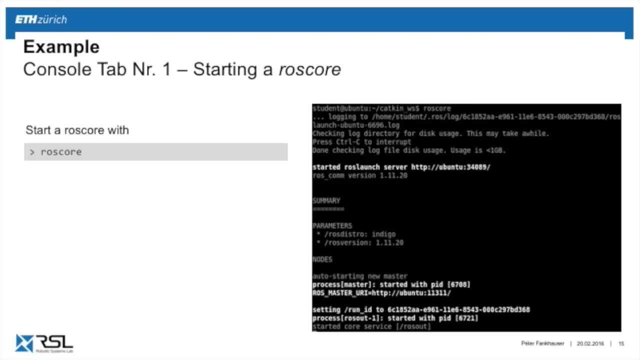 it's not very fundamental but for people who wanna try they can open up their virtual machine and open up a console so we can go through some very, very basic exercises here together. But this is not part of the official exercise, just for trying a little bit out. 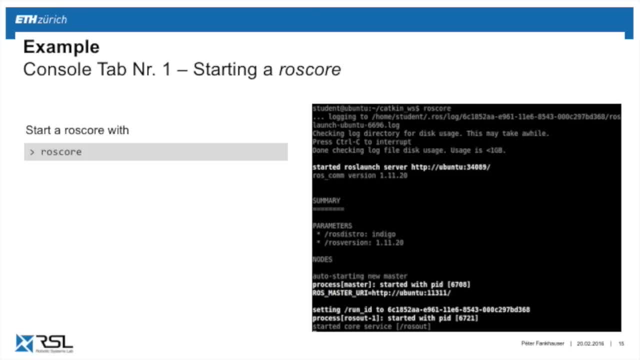 So you can open a console on the left-hand side- It's a little black box Terminator- And then you can create. in one of these consoles you can create multiple views by right-clicking into it and can say split horizontally or vertically. 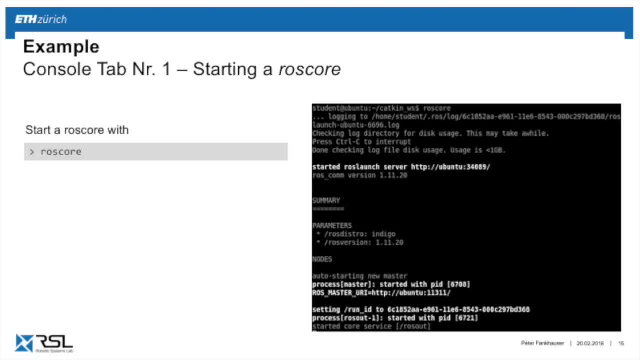 or you can create multiple tabs, And we're gonna use four of these windows or tabs in this exercise. So in the tab number one you can type in ROS Core to start to ROS Core, ROS Master, And you should see the output like seen here. 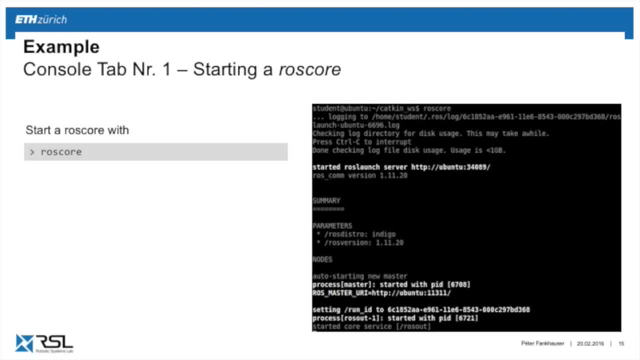 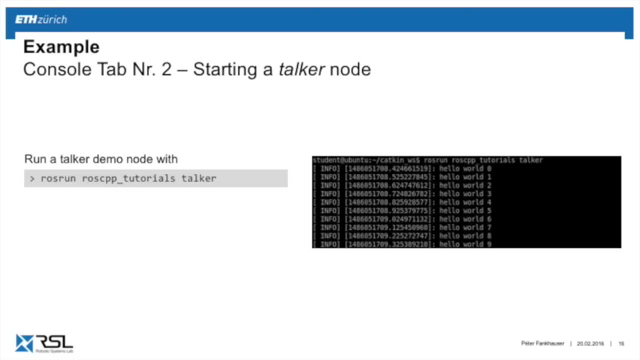 on the right-hand side. Okay, Open a tab, number two- or split the window. In this console we're gonna type in, we're gonna run a talker node which is already a tutorial, which is pre-installed in your system. 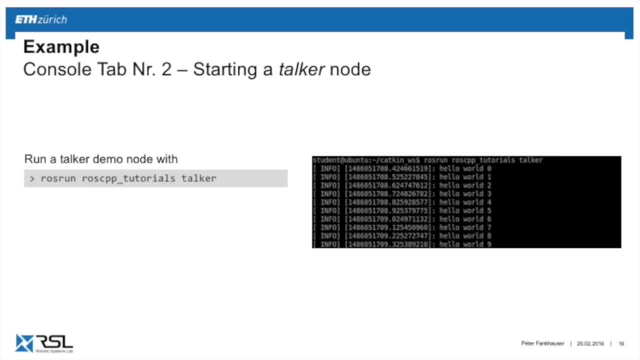 You can type in ROS run to start the node and then ROS CPP on the line tutorials, just a package name and then talker for the node name. Once you are running this node on the right-hand side or in your console, you should see that the node is running. 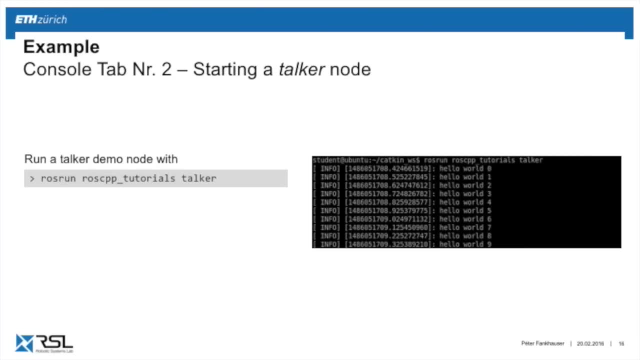 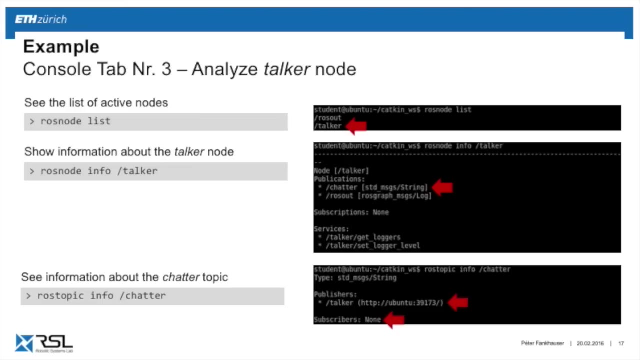 and spitting out hello, world zero. and with an increasing number, essentially this node spit out this message in the console. Now you're gonna open console number three. I'm gonna look at what is happening right now in your system. So by typing in ROS Node List, you should see the node. 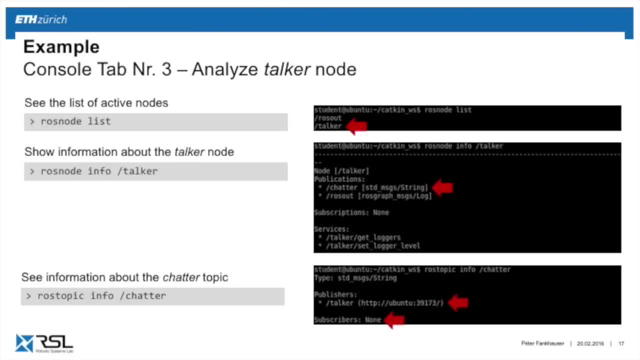 which is just started in console number two. If you do ROS Node List in the console, you should see that you have here here your talker node that you just started. Now, if you wanna know more information about the talker node, 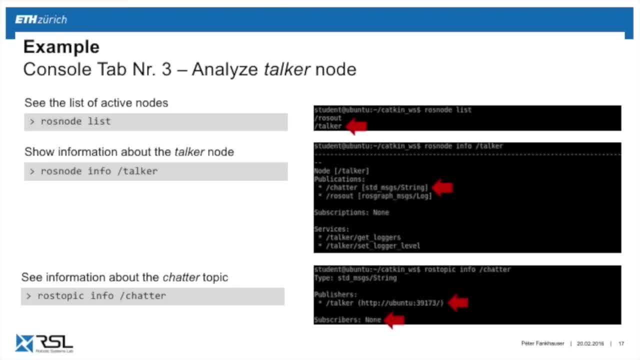 you can type in russnode info, slash talker, which is the name of your node, And then you'll see that you have the node talker which publishes on the topic chatter With of the type string. So essentially this node spits out on your console. 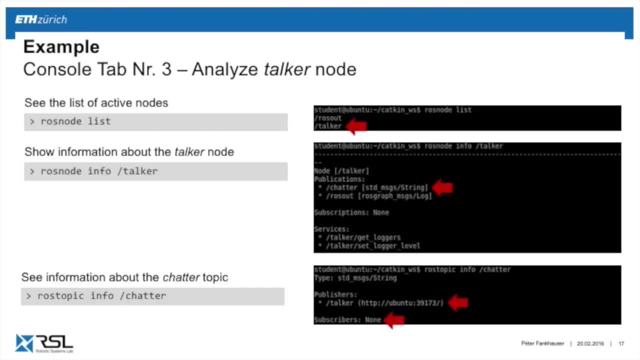 this message, but also provides a topic called slash chatter, where the same information is published to ROS. Now to know more about this topic, you can type in ROS topic info- slash chatter, to see that there's one on the publisher, the talker node here. 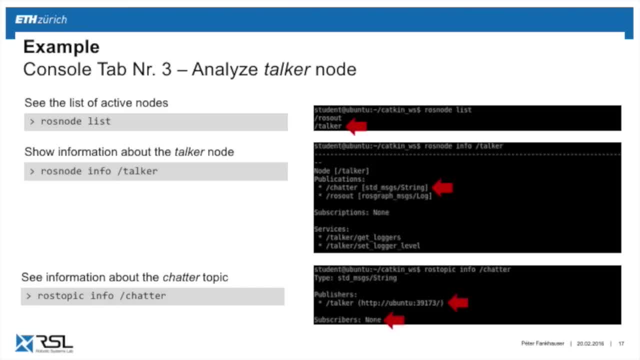 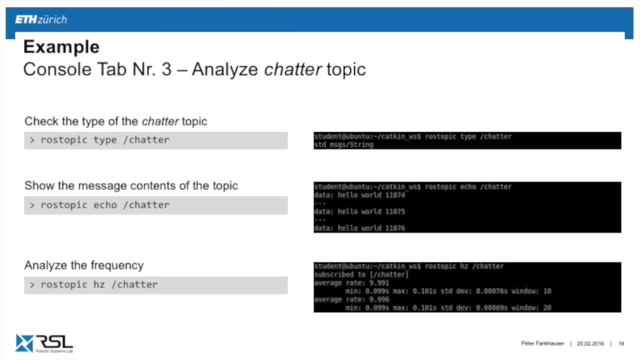 and there's no subscriber yet, So this message is just sent out to nobody yet. So we have started the ROS core. We opened up talker node and we looked at the node, We analyzed it Can look now more closely onto the chatter topic. 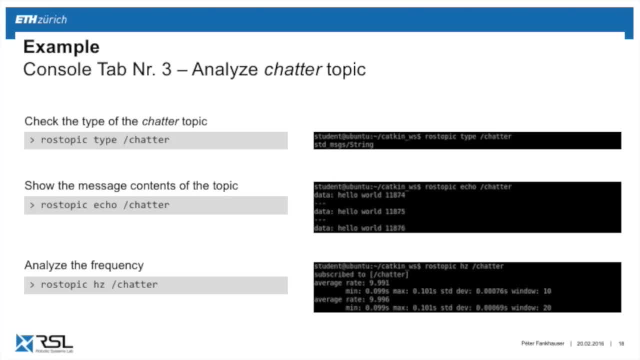 which your talker is publishing. You can do this by ROS topic type and then the chatter which your talker is publishing. You can do this by ROS topic type and then the chatter which tells you: okay, this topic is of type: standard messages string. 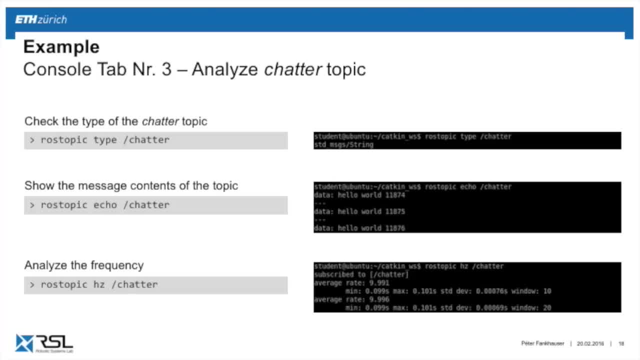 You can look at the contents now of this topic by typing in ROS topic echo slash chatter, which then, similar to your console number two, prints you the contents of this topic into your console. You should see the message going up with increasing number and you can see that it's going up with increasing number. 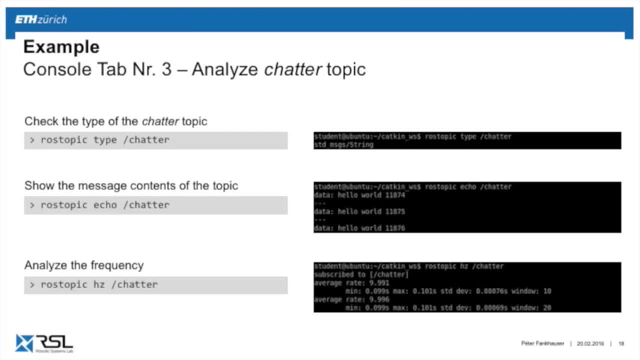 Now there's other commands, such as ROS topic HZ for Hertz, which provides you the frequency of which this topic is published. So if you type in ROS topic: HZ, slash chatter, you'll see that it measures for a while and then gives you the average rate. 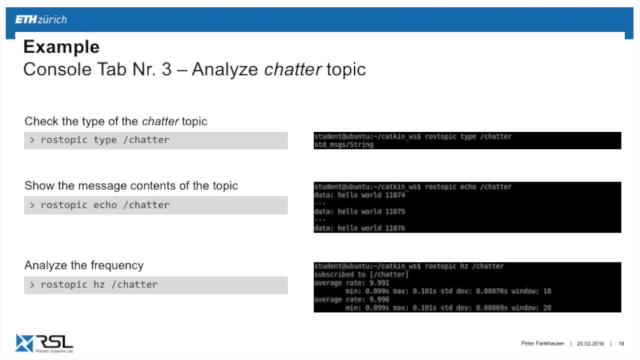 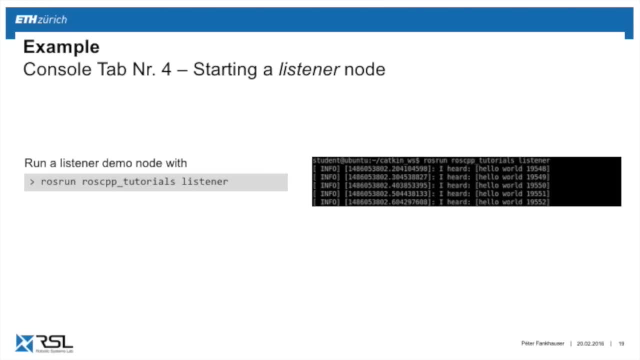 that it would have min and max and standard deviation. How fast are these messages sent out on this topic? Now we have the talker node, It's running, It's publishing on this chatter topic and now we want to start up a listener. 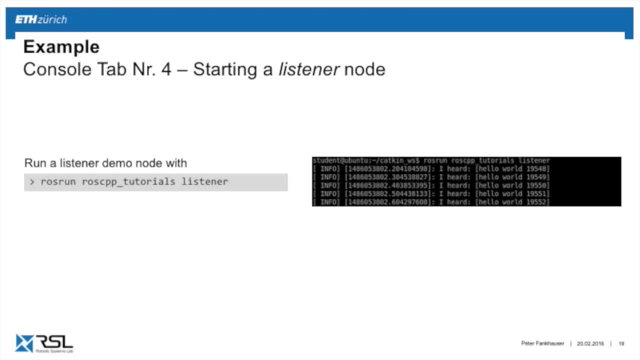 So a node that subscribes on this topic? Yeah, So you can do this by again in console number four, a new console by ROS run and then ROS CPP tutorials, and then instead of talker I will use the listener. 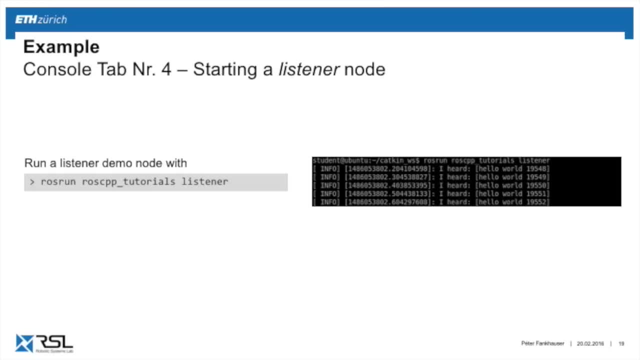 And these nodes already know on which topic the other one is subscribing, Since it's a tutorial, and then you should see now, once you start this node, that it spits out: it says I heard so it's subscribed to this message and spits out the contents of it. 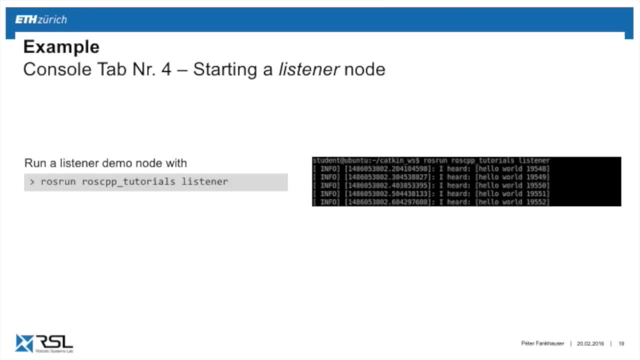 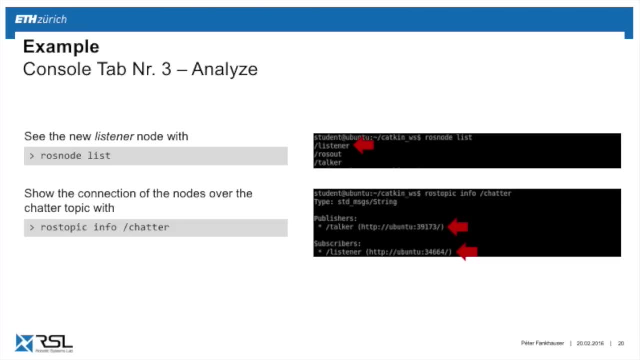 So it says- I heard hello world some number. Now to see that these two nodes are now working together, you can go back, leave them running and go back to your console number three, where you analyze things, And then you can again. 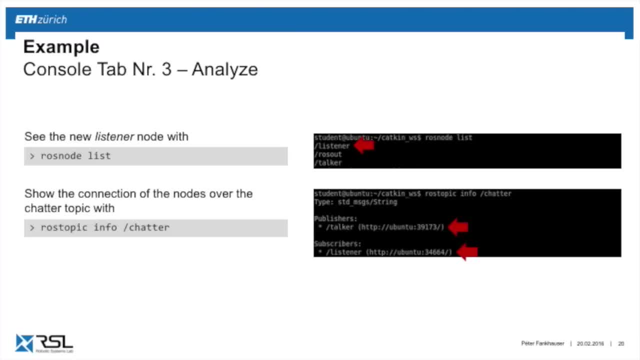 it's the same command as before by ROS node list. Before we only had the talker. Now you'll also see that you started the listener and you have these two nodes running. If you now do the same command as before by typing ROS. topic: info: slash chatter. 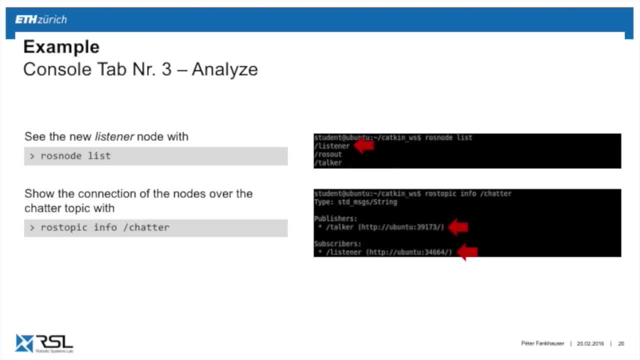 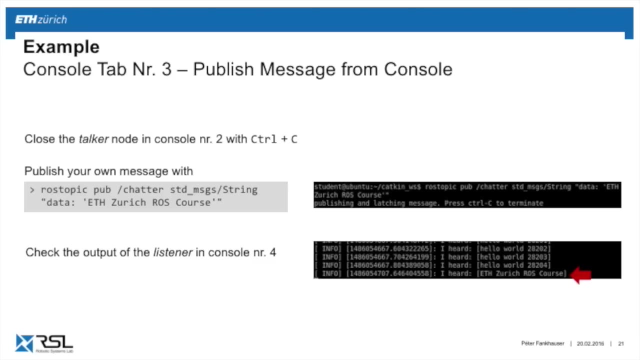 it gives you information about this topic. You see, now that we have one publisher, the talker, and now the newly created subscriber called listener, So these two nodes are now connected through this chatter topic. Now we're going to close the talker node. 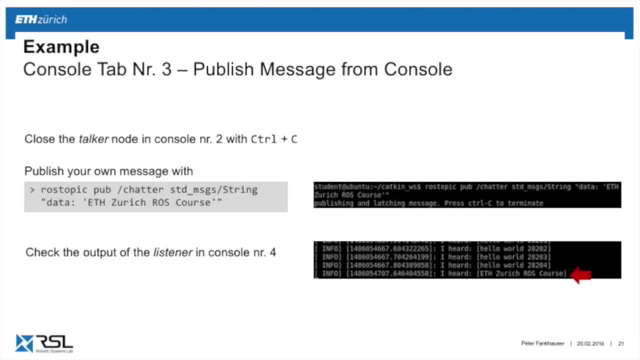 So we lose essentially the guy who gives the information by going to console number two, where you started it, and typing in control C. Then you should see that the listener node stops publishing messages, since it's not retrieving any. What we want to do now is in console number three. 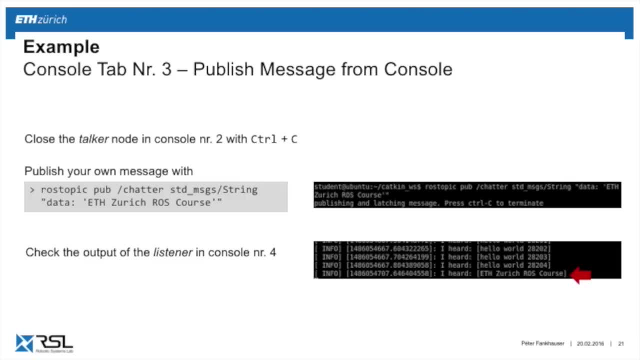 in console number two or three, publish your own message. This is a little bit longer command and you can type in ROS topic hub for publishing on the topic: slash chatter of type standard messages, slash string And then, if you use the tab button, 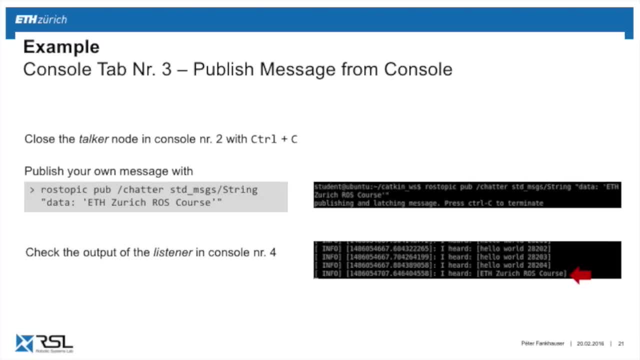 it gives you this structure where you can fill in any message that you want to publish Here. in this example I filled in etagezeric ROS course. Now if you type in this command in console number four, where the listener runs, 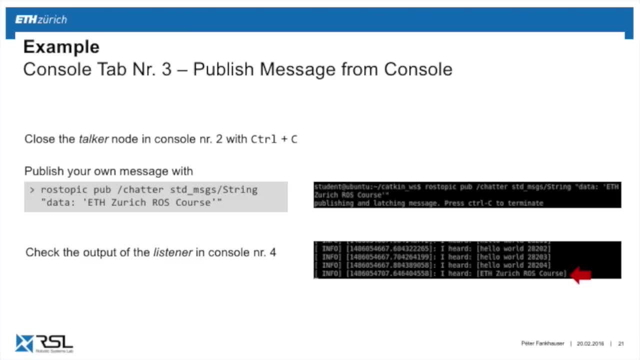 you should see. instead of hello world, it suddenly tells you: okay, this is a message I got, That's the one you published from your console, What you saw, that you can subscribe to topics and show the contents in the console and also you can publish messages from your console. 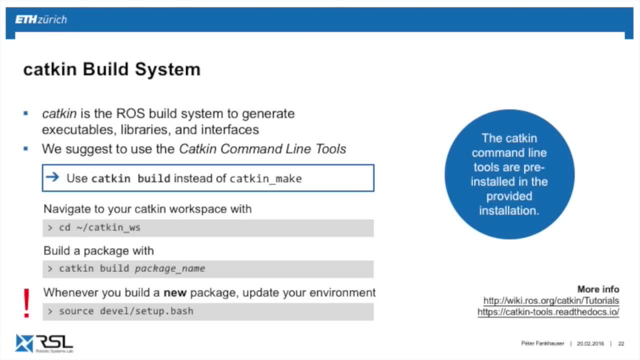 Now we played around with some of the console commands and I'm going to talk a little bit about the ROS build system. Essentially, this is the system where when you write, when you download a package, you write your own notes how you're going to build your executables. 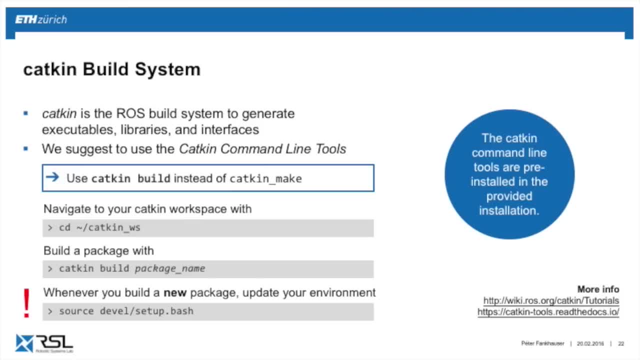 your libraries and the interfaces. The standard way of ROS so far has been the catkin make command. We suggest the much better tool, the catkin command line tools. This is already pre-installed on your system. It's very similar. 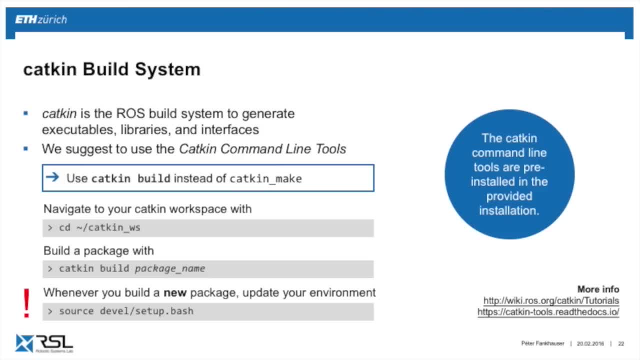 However, it provides nice functionality. So whenever you see in a tutorial on the web catkin make command, it's important to type in catkin space build instead of catkin underline make. type in catkin build, which is fundamentally the same thing. 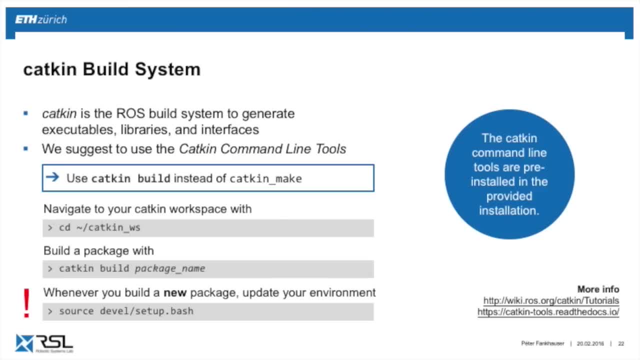 but don't mix these two commands. You're going to have a lot of problems. You're going to have a lot of problems. I suggest you use catkin build command and the commands that I'm going to show you in a second. okay. 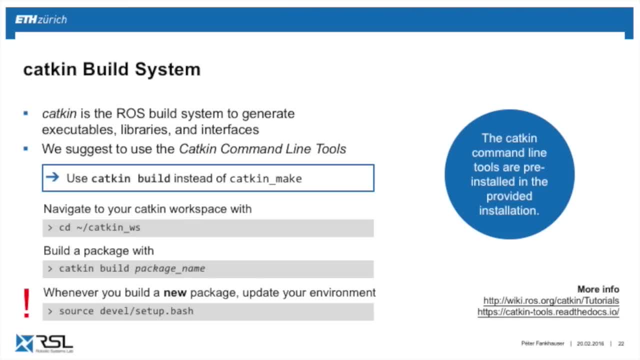 So you can. typically, when you want to build a node, you would have to go to your catkin workspace by CD and then going into a catkin workspace And then you can build a package by catkin build and then the package name. 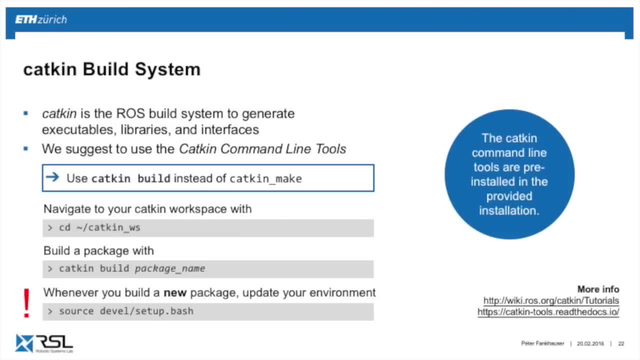 Now here's a very important part: Whenever you build, whenever you build a new package, your system should know about it, must know about it in order for you to use it. So you have to resource your console. You can either open a new console. 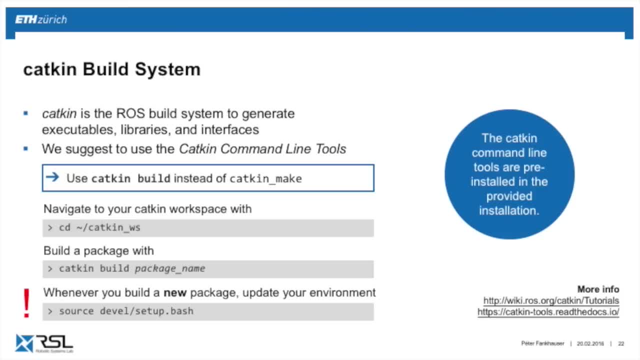 but it's simply, you can type in source And then, if you're in this folder, devil folder, slash, setup, dash, this scans again your environment to make sure that your new node, that the system is aware of your new node, your new package. 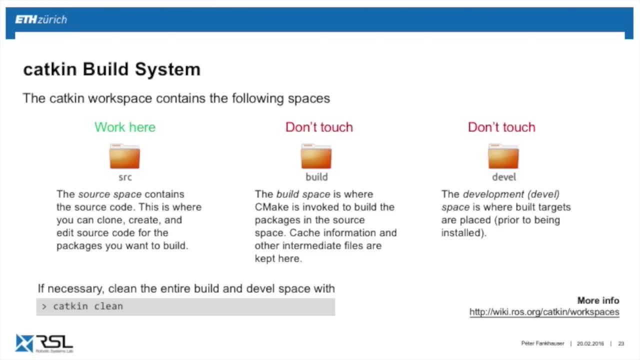 Now, once you build your catkin workspace, you'll see that you have three folders in there. One is the source folder, a build folder and the devil folder. The source folder is where you put all your source code information, and the build folder is essentially a cache. 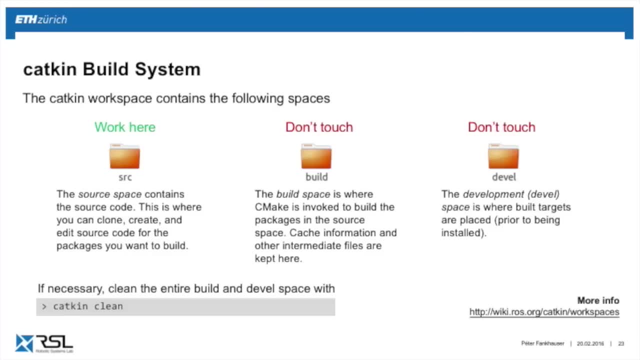 folder for the CMake folder, CMake system. And the devil is where it puts the executables before, if you install them, before installing them for you to use Now. these two folders are taken care of by the catkin build system. 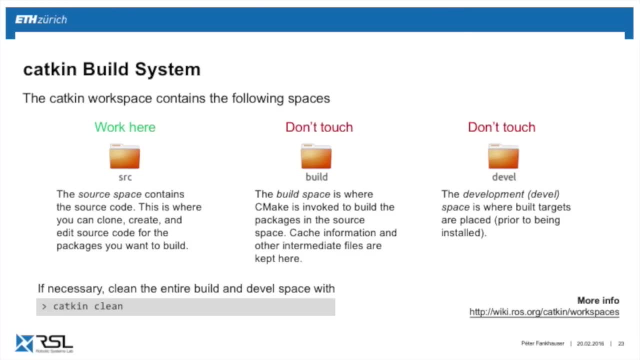 I put all the information there and make sure it runs. So you don't typically never touch these two. You do all your work in the source folder, where your source information is stored. If you run into troubles, ones that something is mixed up. 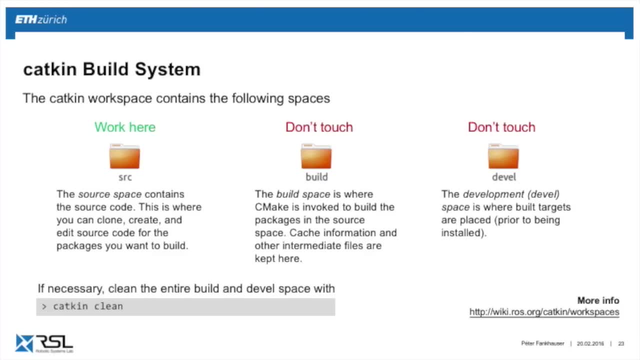 you change too many things and you're not sure you want to build from scratch, you can type in catkin clean which wipes out the build and the devil folder. It doesn't touch your source folder, but then you can rebuild from scratch again. 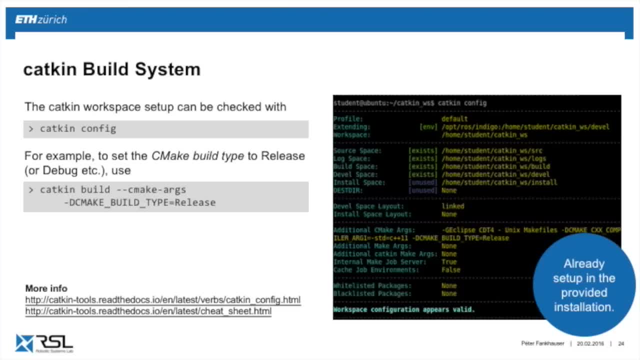 There's a setup associated with your catkin configuration and you can look it up by typing in catkin config In the virtual machine that you got. we already set up And if you type in catkin config, you should see this output. 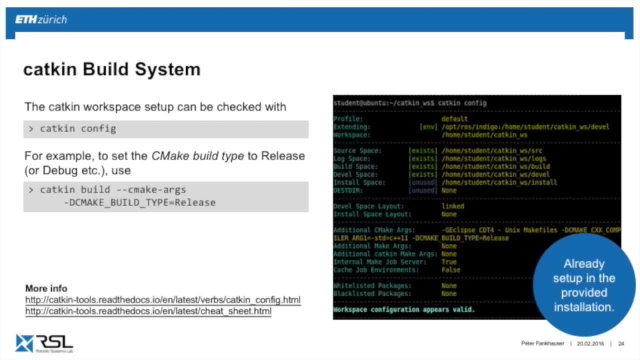 One of the important parts are these CMake arguments. We already set this up for future reference. You can set them by catkin, build and then CMakeArgs, and then you type in all the arguments that you need, For example, if you want to build in debug or release mode. 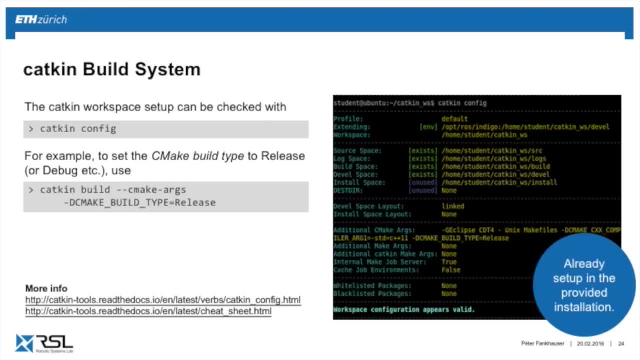 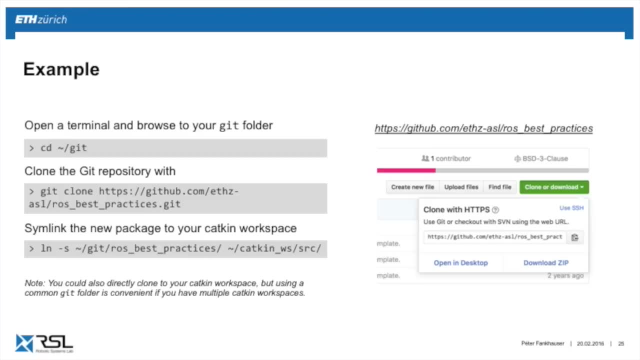 if you want to create the Eclipse project files, et cetera. There's nothing for you to do right now, just so you know in the future. Now we come to a second example, And what I'd like to do is go. 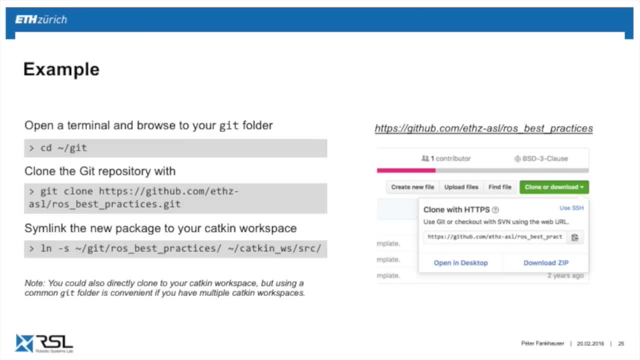 say, on a typical GitHub website and make you download, clone a Git repository. This is a typical tool that you'll see when working with software, And then we're gonna build this on your system So you can go on the website githubcom. 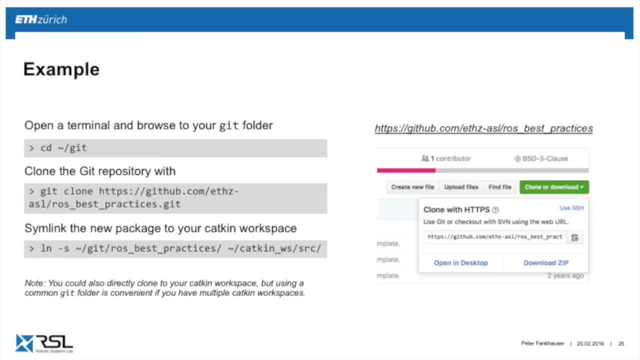 slash E-T-A-Z minus A-S-L. slash ROS best practices. We put up there an example ROS package for you to play around with. Now I'm gonna go to the top of the page and I'm gonna say: clone this. And I'm gonna say: clone this. 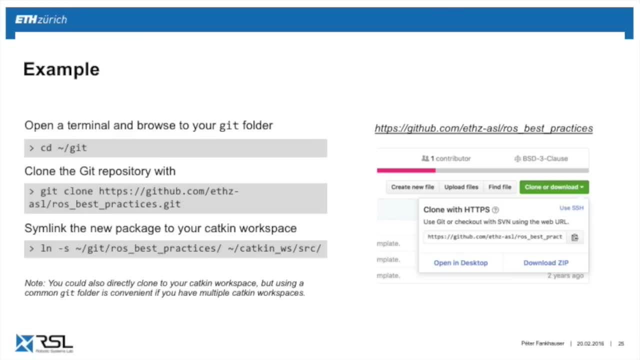 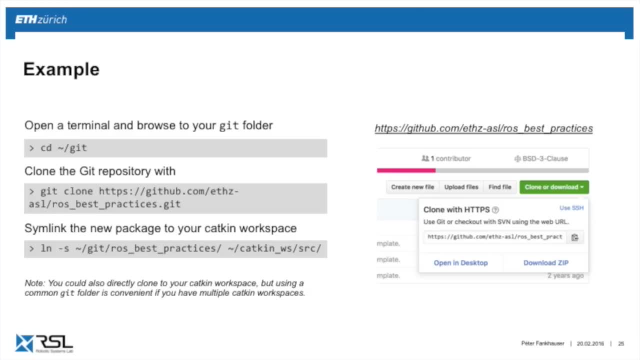 And copy this URL here. Then you'll see in your system that you have a Git folder. Just go into CDs from your home folder. you go into CD Git And this is where we're gonna clone now The software. cloning means actually downloading the software in a Git format. 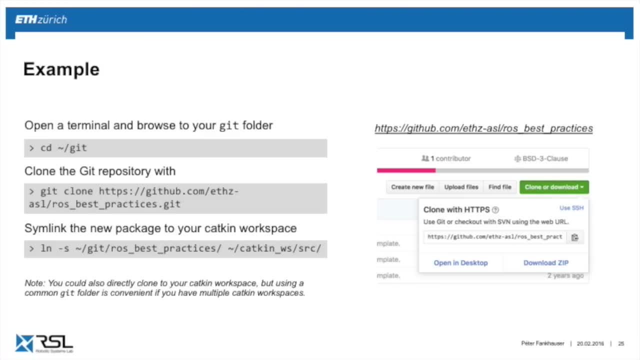 You can type in Git clone and copy paste the URL In a console. you can paste by control shift V. So instead of just control V, you type in control shift V. If you press enter, this will clone all the information from this repository into your system. 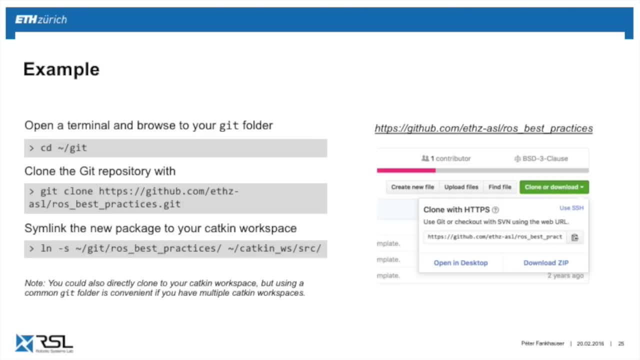 Now you've seen that we put this into the Git folder. It's nice, if you have multiple workspaces in the future, that you have one main folder where you store all this when you clone all the software. So that's why we put it into Git. 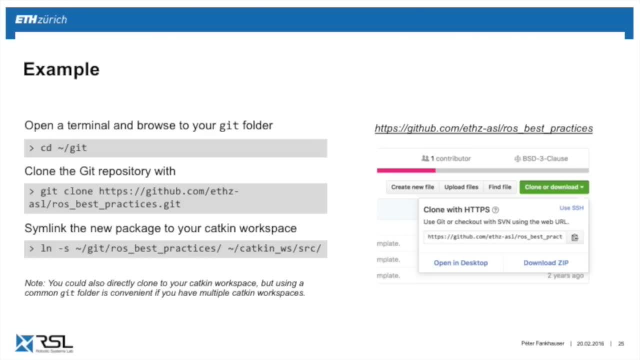 And then what we're gonna do now to work with it. you'll have to save it. We're gonna link it into your catkin workspace. You could also directly clone into your catkin workspace, which we recommend you to put it first in your Git. 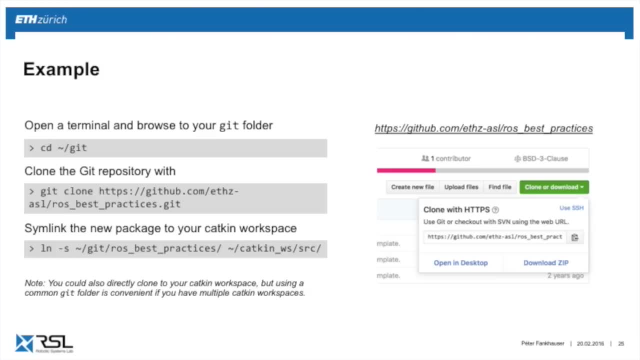 and then sim link it into your catkin workspace. Now, to sim link it, you would type in LN minus S to create a symbolic link and then tell it from where to where. So in this case you would say in the Git folder: 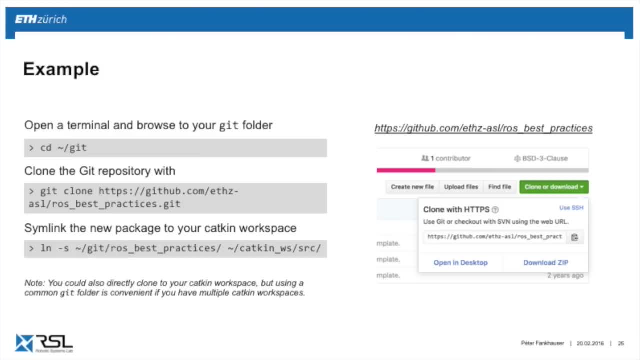 the ROS best practices you wanna link into your catkin source folder. Now, after sim linking, you should see in your catkin slash source a folder: the ROS best practices folder. Now, once you have cloned and sim linked it in your catkin workspace, you can go to your catkin. 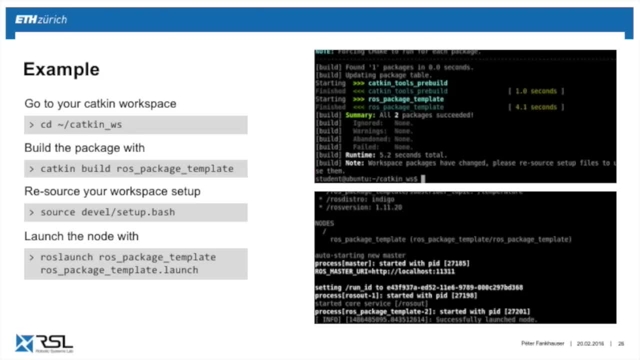 workspace by CD catkin workspace And then use the build command as we saw before, by typing in catkin space build space ROS package template. This is the package which is stored in the Git repository. What you should see is what you get here on the right. 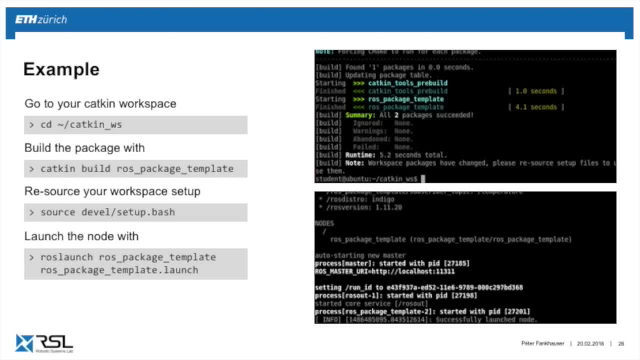 head side is that it builds these and it shows you information how long it took. Now, since we downloaded, we cloned the new repository and now we're gonna do the same thing Once you download the new repository. like I said, you need to source your workspace. 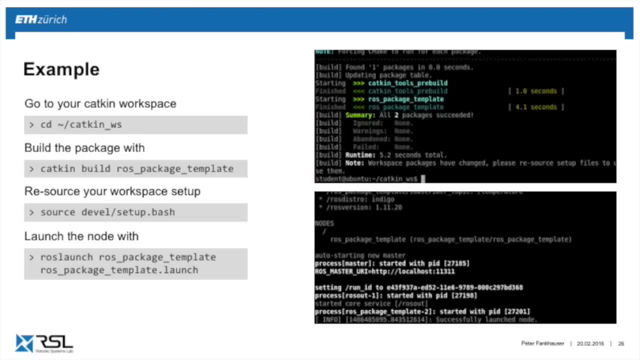 You need to inform the workspace that you have something new. You would type in source slash devil setup dot bash. This is an important step And if you find yourself at some point that your catkin workspace doesn't find your package, just type in this command again to make sure. 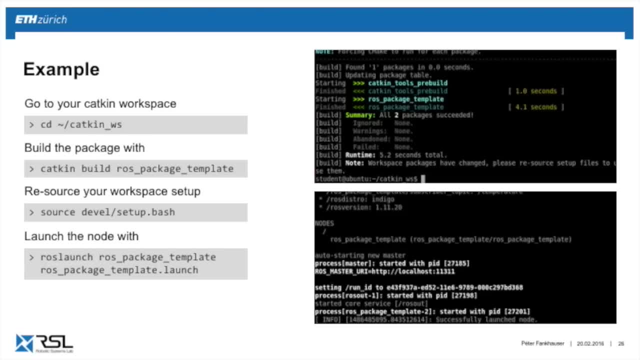 that all the information is up to date. Now we have clones repository. We've built it and you can start it now. We haven't seen this, but we'll see in a second. Instead of ROS run, you can do now ROS launch. 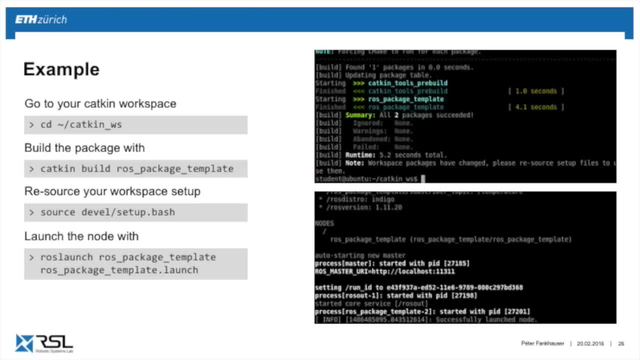 which is a similar topic, and we'll see what the difference is. So you can do ROS launch and the ROS package template, which is the package name, and then ROS package template dot launch, Which is the name of the launch file that you use. 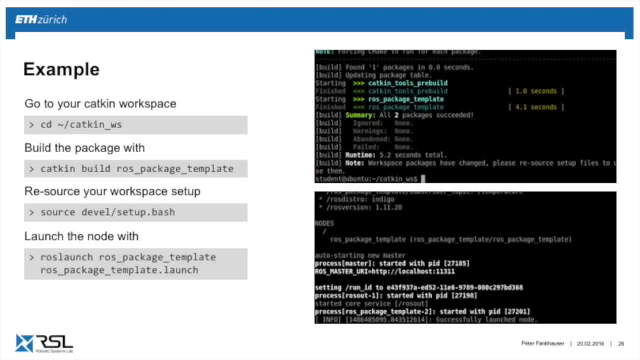 If you type this in and again use the tab command to make it very quick, you should see a ROS core starting and two nodes, or one node actually starting and saying successfully launched the node. So if you go through this, you've. 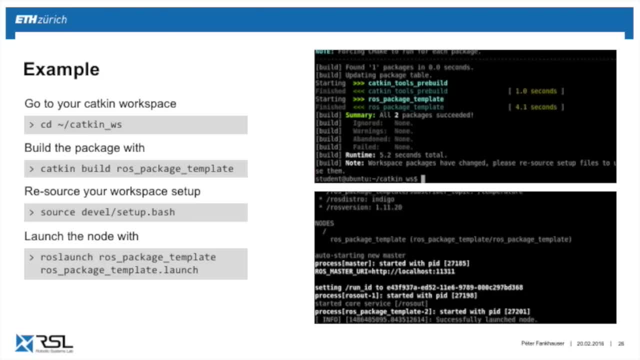 seen that you can take source code from the internet, clone it, build it and run it. These are all the necessary steps that you need to do to do that. Yes, Can you go over this again for me, like first? OK. 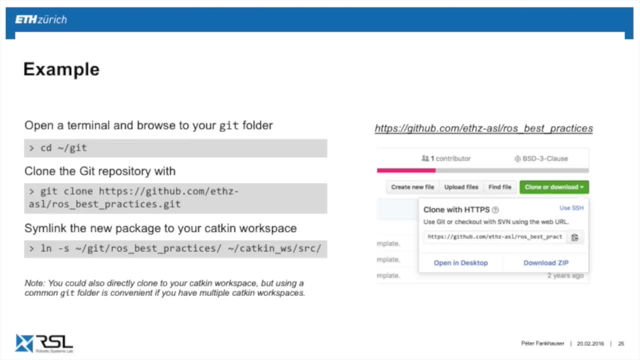 So what we did is you can have multiple workspaces. So this Captain workspace you have now only one in your system. In the future you'll see you might have multiple. So if you work in this class, you might have a semester thesis. 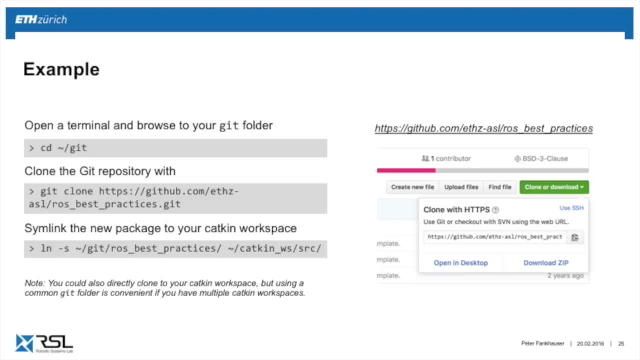 You don't want to mix too many of them. So to keep it clean, instead of every time once you need a package, cloning it into the Captain workspace, what we recommend is to create one central Git folder. From there you can symlink to the different Captain. 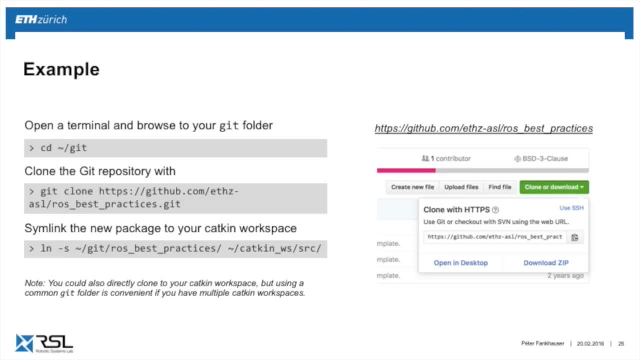 workspaces, only the ones that you actually need in your Captain workspace. In this example, you could also as well do it just directly in the Captain workspace. It wouldn't matter technically, But in the future it's nicer to organize your system this way. 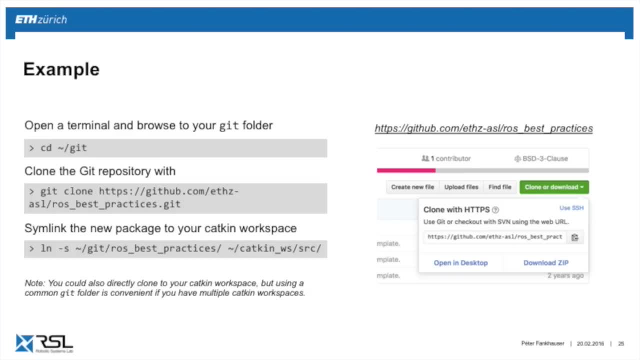 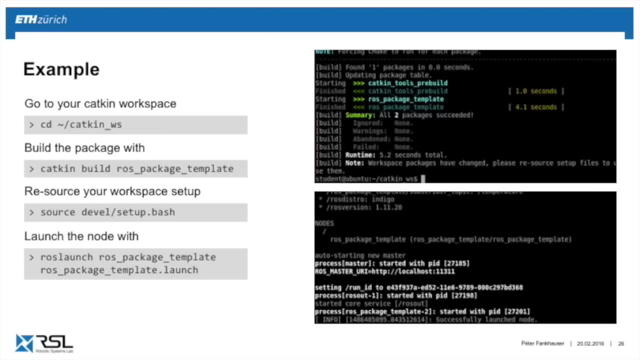 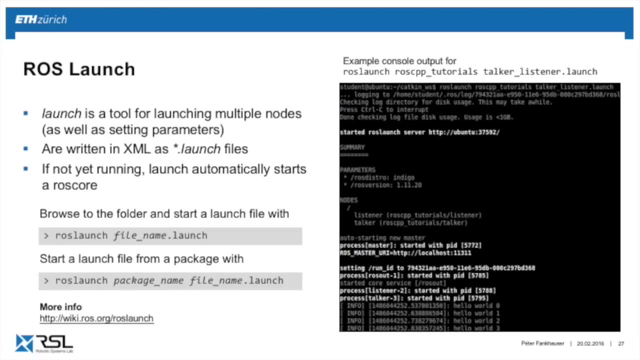 That's why we show it this way. Does that make sense? Yes, OK. OK, so you've downloaded, built and launched software for ROS, And we saw in the last command that you used ROS launch. Launch is essentially a tool to run instead of typing. 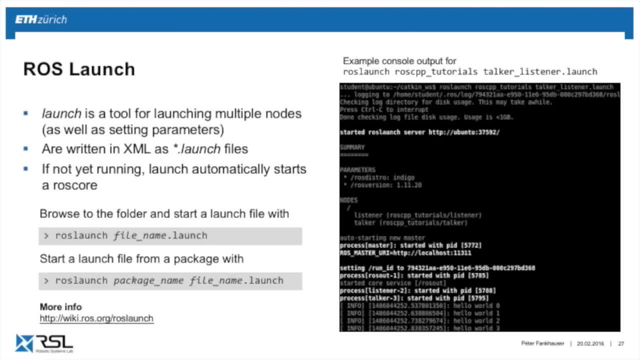 every time in a console ROS run, You can combine them in one launch file which informs the system which nodes and which information does it need to load. It's a very convenient tool to run your system, These launch files, and this is important. 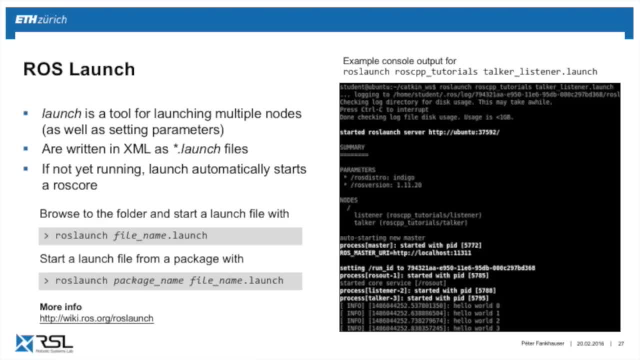 you'll write one in the exercise are written in an XML language and are stored in launch files. Also, as a side note, if not yet running a ROS master somewhere, launch automatically will run this for you. It means you can go into a console. 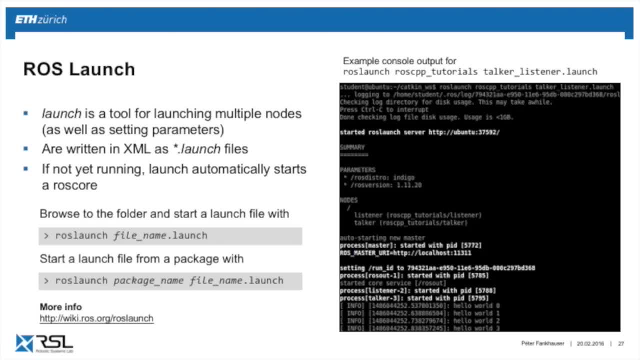 type in ROS launch- the launch file that you need, and it will boot up everything that you need To start a ROS launch file. like we already did, you would type in ROS launch and then the name of the launch file If you already have a package, like we had before. 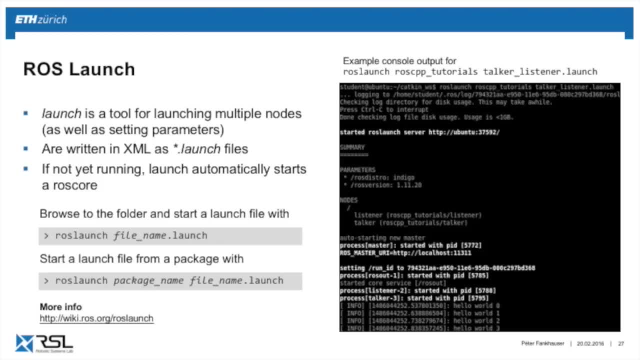 so in the first case you would need to be actually where you launch it. You'll have to be at the path where you want to launch the launch file. If the launch file is associated with a ROS package, you can type in ROS launch package name. 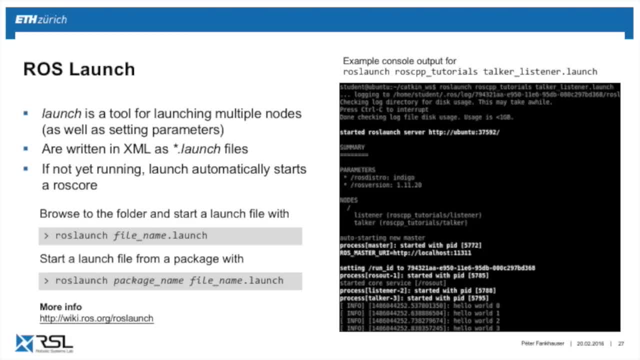 and then the launch file, such that you don't need to be at this path of the file. It finds it for you automatically. If you want to type in another example, you could do like we had the talker and the listener before. 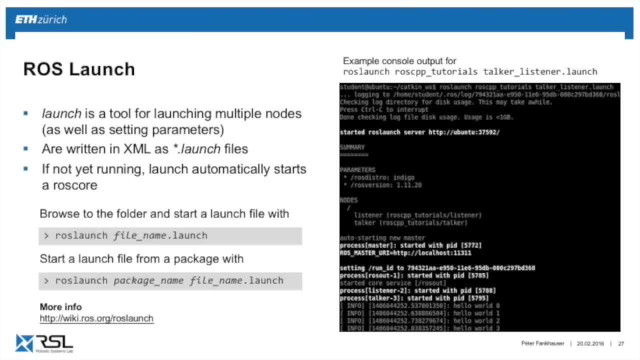 There exists a launch file which launches the two together and you could use by ROS launch ROS, CPP tutorials and talker listenerlaunch. This guy does the same work you did before: starts the talker and the listener together. Now, if we look at this listener and talker launch file, 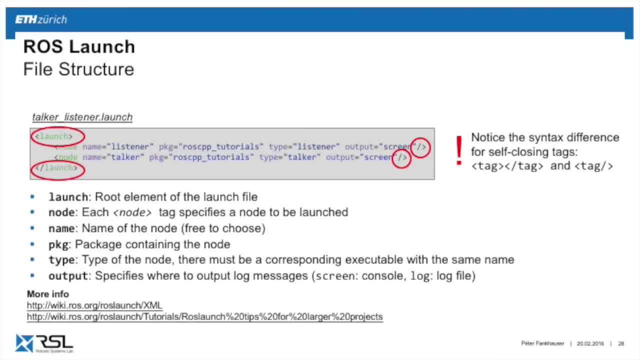 this is how it looks like. You have, in the bottom and the top you have a launch XML tag And then you see that We have two lines to start: the two nodes. Each node's tag line specifies which node to run It has the parameter's name. 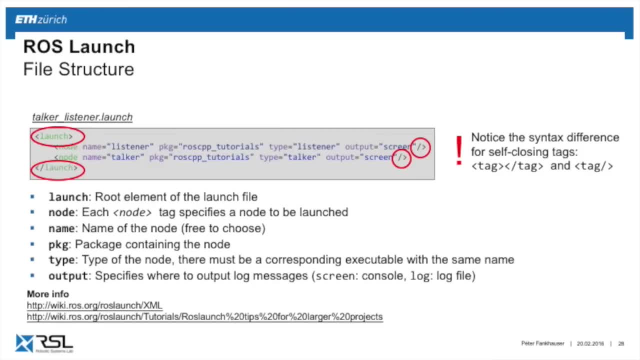 This is an arbitrary name that you can choose to run under which name you want to run the node. And then the PKG, the package name- In this case it's a ROS, CPP tutorial- And then which executable, the type. In the first one, the listener will be of listener type. 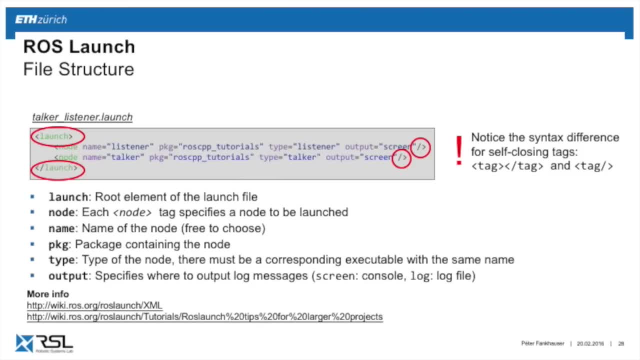 And the second one. the talker is of talker type. The output information at the end tells you on where to put the information that it provides. In this case we say screen, which means you print it on the console, But if you want you could also say log. 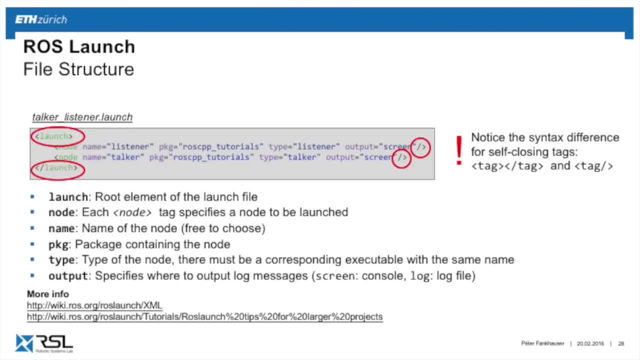 to put it in a log file. if you don't have access to that console, It's a convenient tool to debug. Now, very importantly, once you write your own launch file, you see the difference between here a closing XML tag which launch, and then this sign to close it again. 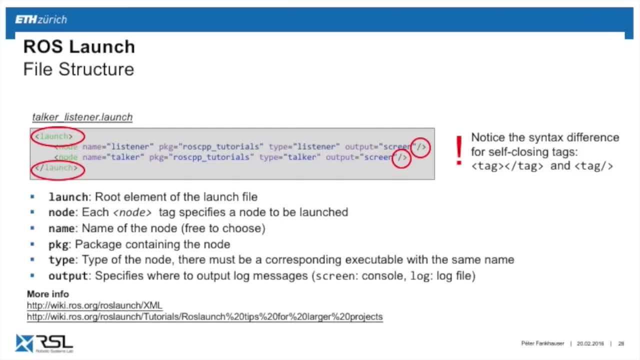 And you have self-closing tag, XML tags such as this node, which in the end has this slash on the very end. They mean the same thing, but one is self-closing and the other one can contain elements. So whenever you'll see an XML error, make sure. 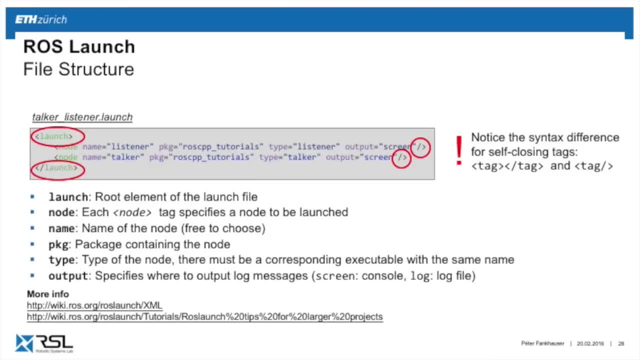 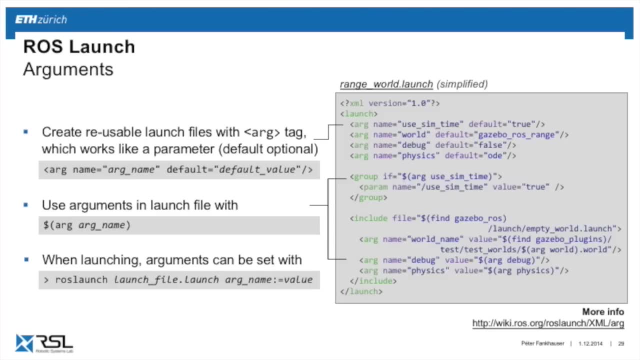 make sure that you have these tags correctly. Now here's another launch file on the right-hand side. One of the nice things is you can, once you build up a nice launch file, you can reuse it with different parameters. This is where the argument tag comes in play. 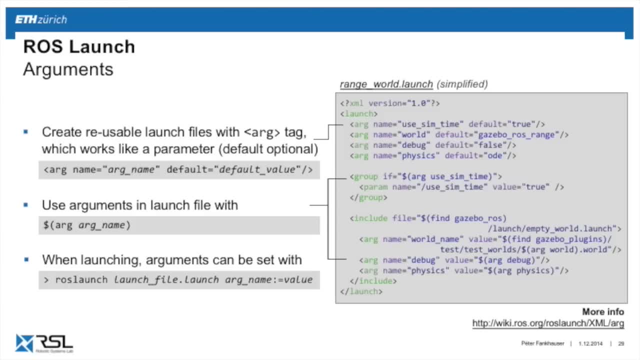 So in this example it starts a simulation and has four tags, four arguments saying use simulation time, which world to use, use it in debug mode or not and which physics engine to use. Specify them on the top, like there: 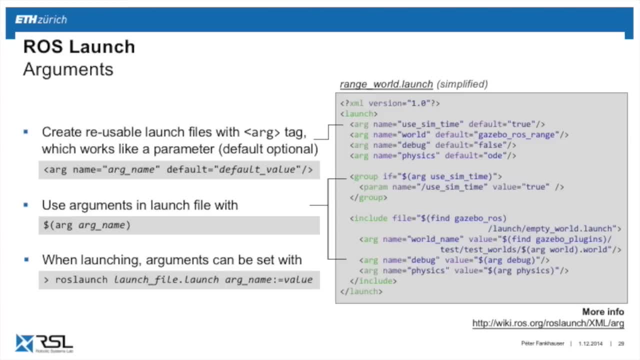 and then you can reuse these arguments in your launch file. So in this case it says: if, if I want to use this argument, if this argument is set to true or false, then also set this parameter And whenever you so, if you specify it up here. 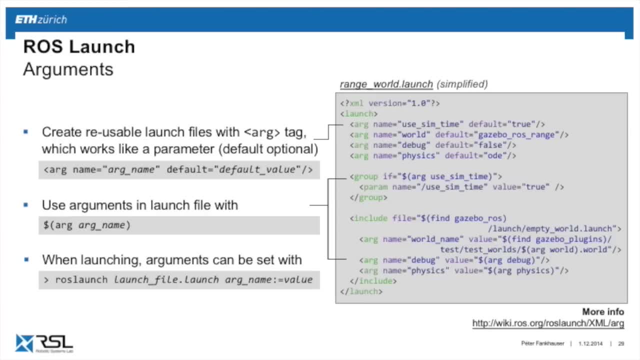 you can reuse this, this argument, by the dollar sign and slash bracket argument and the argument name, which in these two examples also down here. One of the nice things is, once you've set up this arguments, you can launch your ROS launch file by ROS launch. 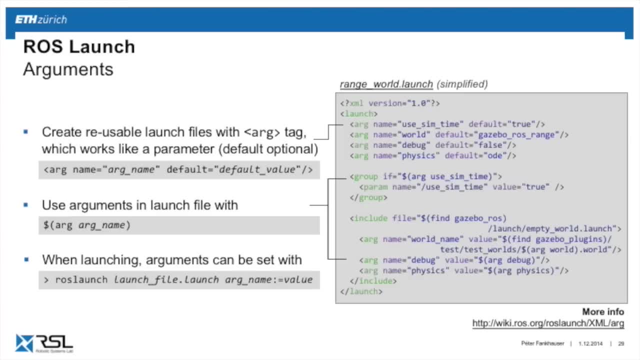 the launch file and then saying: argument name: double point equal the value. So you can use the same launch file from the console saying: once I want to use the ODE physics engine or I want to use the bullet physics engine, turn on and off different elements. 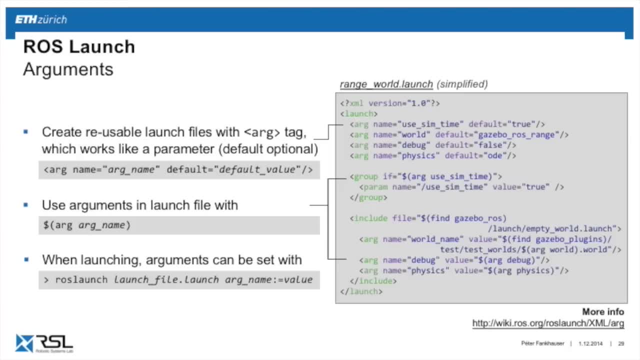 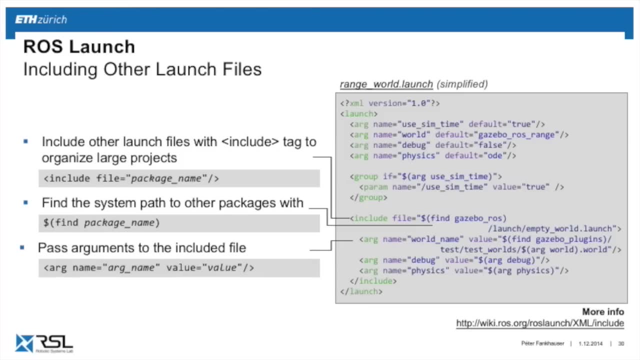 It's a very convenient way to quickly start a certain setup of your node. This is also an important element. You can nest launch files, So in this example you'll see that it uses this include tag and then the file. In this case we want to include. 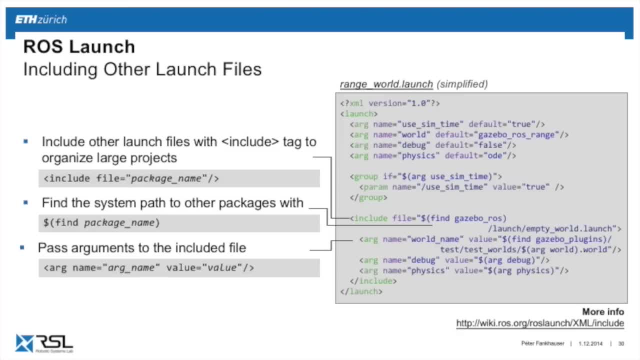 this empty words of launch, which launches an empty world in simulation. It doesn't matter. Importantly in ROS, don't use absolute file path, So if you give it to a friend it might have a different username, et cetera. 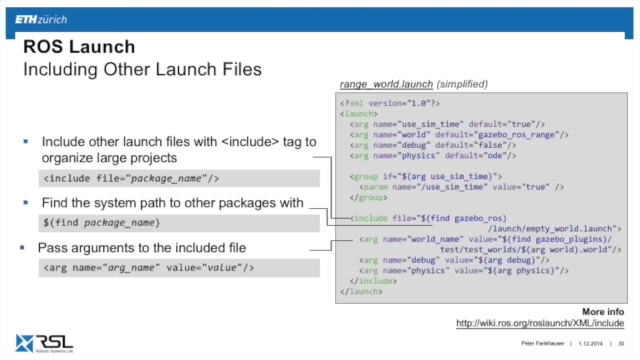 So what we always do is related to a package. In this case it says find and then the package name written here. this gives you the local absolute path And then you would be in the launch folder, the empty word launch Now, if this other launch file. 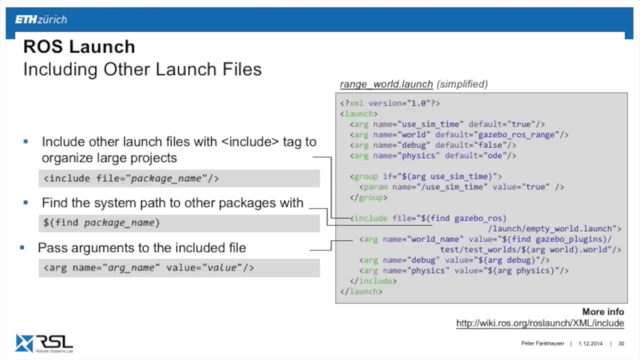 also needs arguments. we can pass them down by typing in the argument name and then the value. So in this case we saw that the name would be for debug- Yes and no would be okay, The name debug again, and the value is the argument that I got from up there. 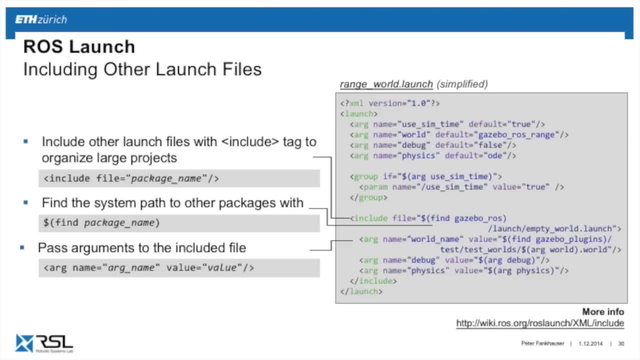 So you can pass down the values of the arguments one launch file to the other one, And by including nesting multiple launch files you can create complex systems that can be launched individually but also all at once passing down the arguments. Any questions to the launch file? 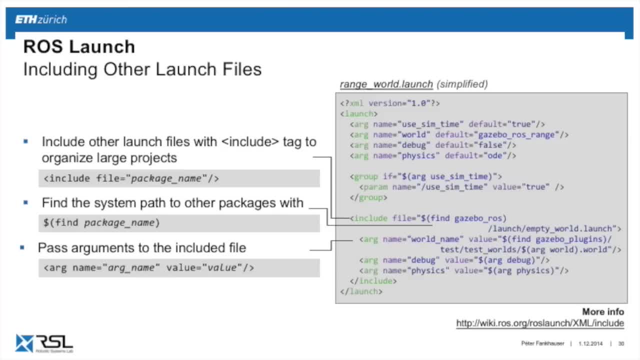 You're gonna need this in the exercise: Make sure that you make the XML structure is valid, and then you're gonna use the include and the arguments, et cetera. Now, one of the elements that we'll play around with is the Gazebo simulator. 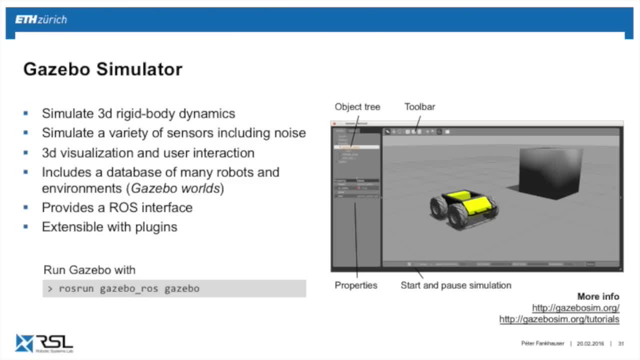 It's a 3D simulator for rigid body dynamics and you can include robots, objects et cetera. It's you can also simulate sensors. You'll see that in a second. So this Husky can carry a laser sensor, for example. 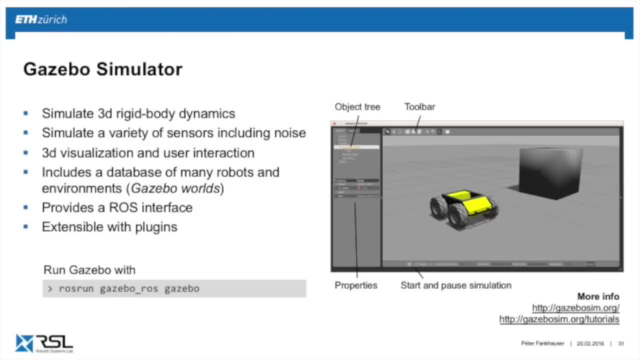 It provides a 3D visualization which is also interactive by meaning. you can have a toolbar up here where you can drop in elements such as this box In the left-hand side. you would see the objects that you dropped. 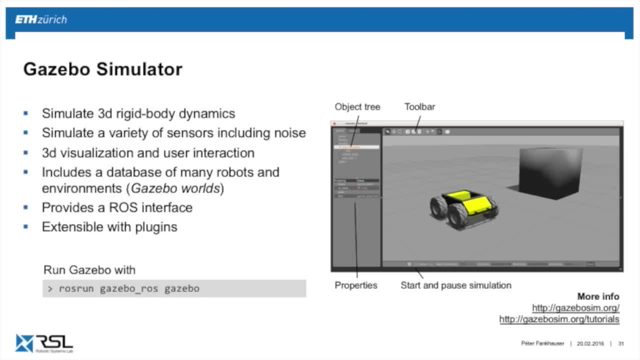 and the robot and, importantly, down here you can start and pause your simulation or slow it down or accelerate it. Gazebo has a database of many different robots, and this Husky robot is a standard robot that comes along with ROS. 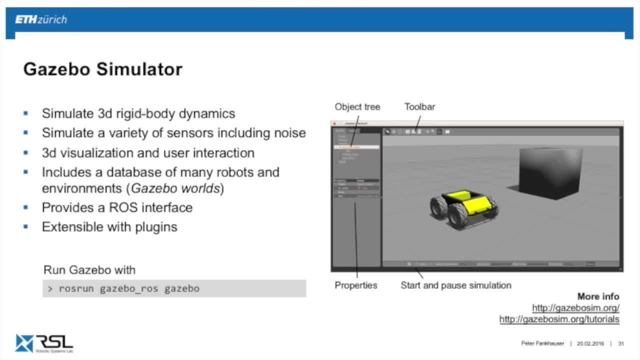 And Gazebo is essentially a standalone program, but it comes with a ROS interface And the nice thing is: in the future, if you want to write your own robot, your own sensors, you can include it into Gazebo through plugins. 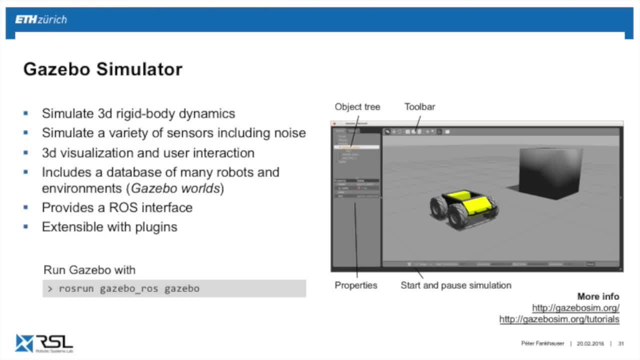 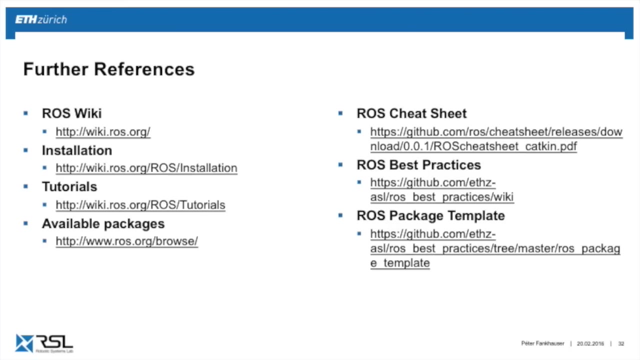 To run Gazebo, you would type in ROS, run Gazebo ROS, which is the ROS version of Gazebo, and then just Gazebo as a node which opens standard empty Gazebo environment. This is the end of the first lecture. 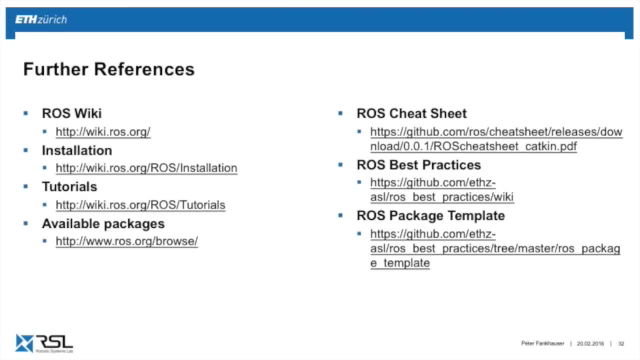 There's for you in the future and now. if you have any questions, you can either ask us, but the internet is full of information. The most important website is probably this, wikirosorg, where they have documentation and tutorials on each of these topics that we talked about. 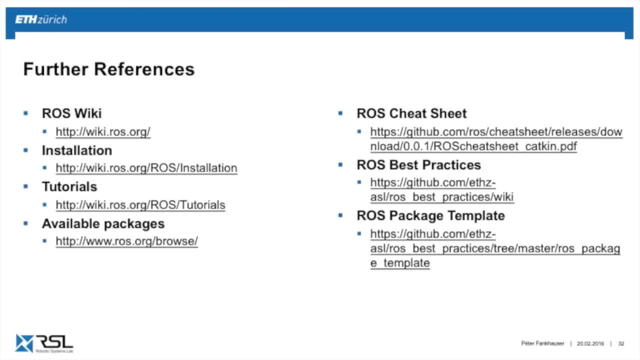 And then there's the installation website of ROS and here's the tutorials. And you don't want to in the future, you don't want to reinvent things. so before you start programming something, make sure that you check it out, check it out, check it out. 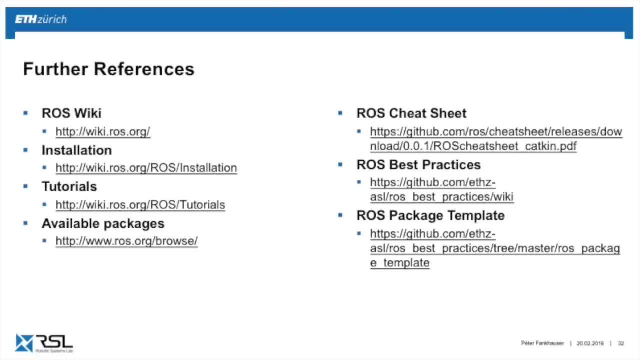 and you check out the existing software. You can do this on the ROSorg slash browse website where all the ROS packages are listed. There's a ROS cheat sheet if you need, but you get very quickly into it and you know them by heart. these comments. 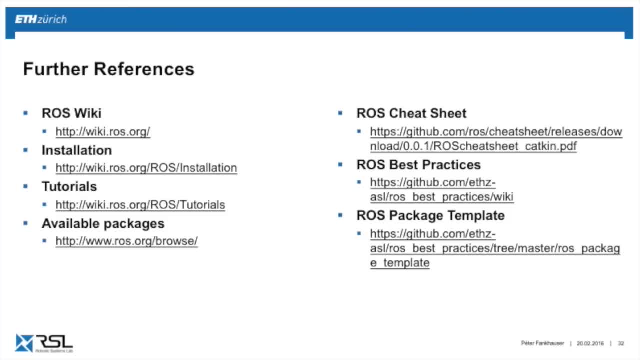 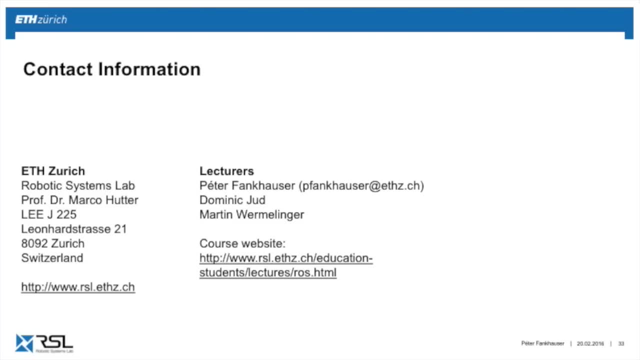 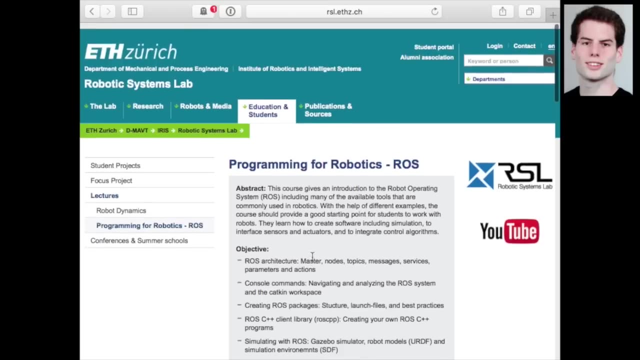 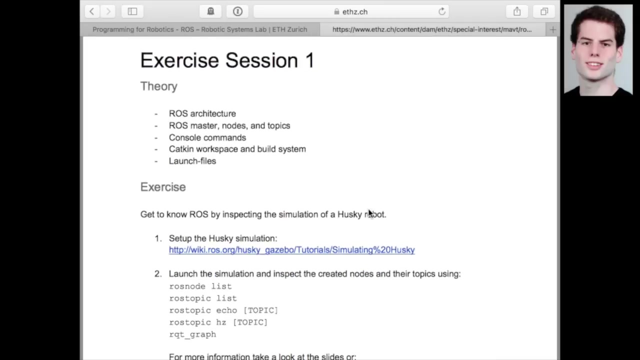 And for tomorrow we'll have two more links that you'll use, or in the next course. Then we'll have Dominik explaining you exercise number one. 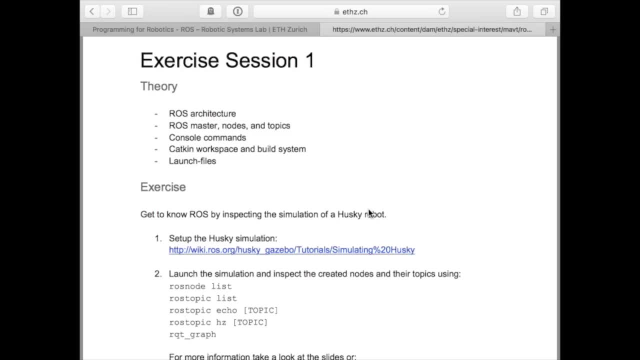 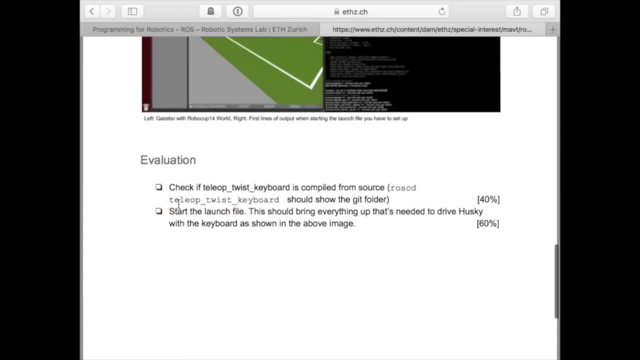 at the very end there's an evaluation. So check these points here. You always see that there are. there's a percentage of how much every point in this simulation counts. Every exercise has 100 percent and there are five exercises so you can get it most: 500 percent. 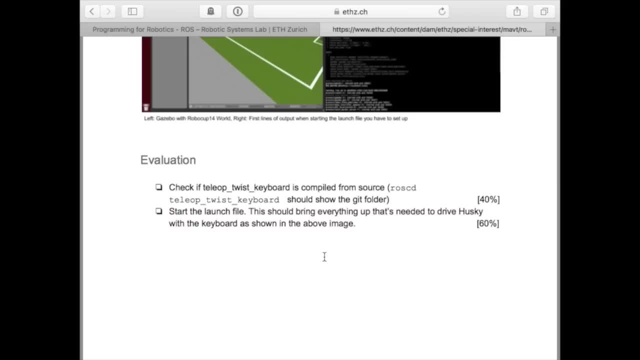 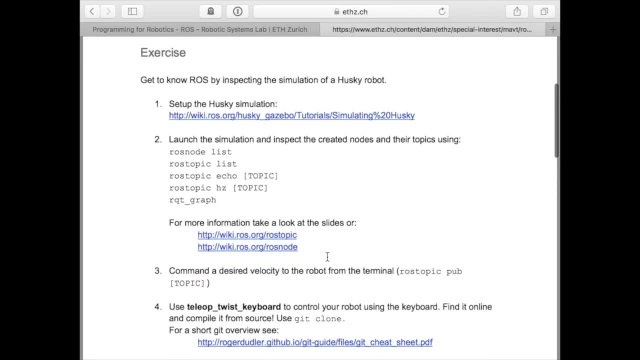 Yeah, so let's start at the top. The goal of this exercise is that you get to know the ROS environment by first inspecting the simulation of a husky robot that you've seen before. You can set up the husky simulation with the link that you see here. 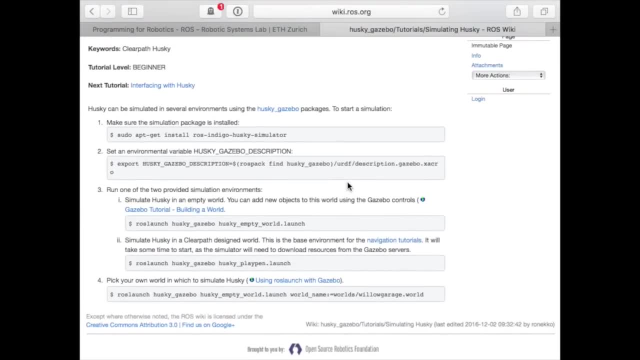 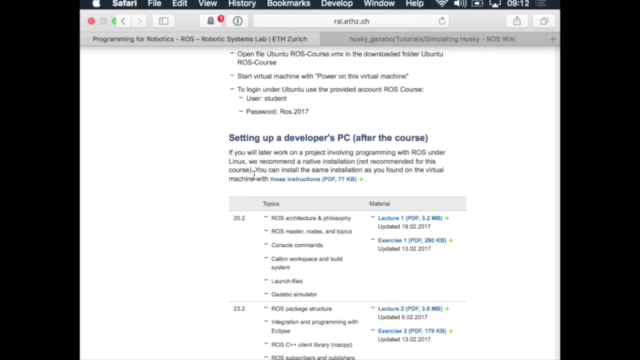 There's a good description of what you have to do to get husky running, And so this only starts: Husky in Gazebo, nothing else. So there's no controller, no lasers, no IMU, nothing, Just Husky in the simulation. Then play a. 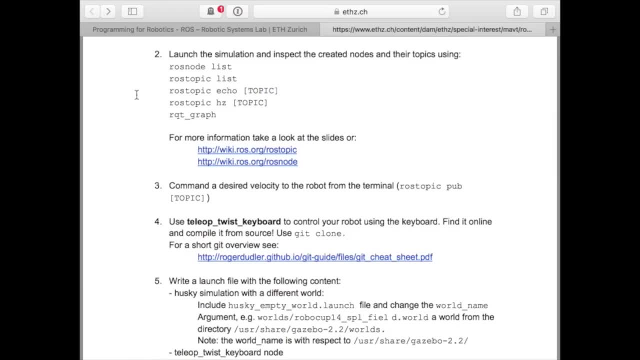 little bit around with the ROS node and ROS topic commands, such that you can really inspect what's going on. So see the topics, take a look at what are the nodes that are created, what is the setup, how do they interact and communicate? 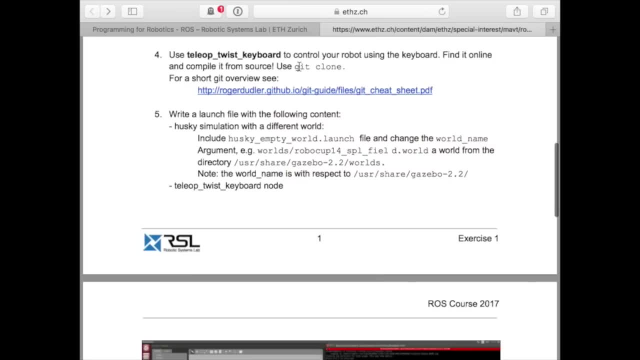 Then clone the Teleop Twist keyboard. So, as I mentioned before, there's no controller running. but with this node you can steer around the Husky with the keyboard, And you could install this from a PPA or you could install it from a PPA, or you could install this from a PPA, or you could. 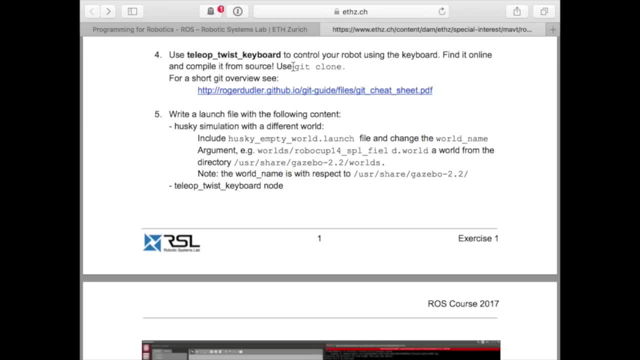 clone it. What you have to do is you have to clone it from Git, as you did with the ROS best practices, and then build it from source. If you need a Git cheat sheet, then there's a quick link that you can press on and you'll just see. 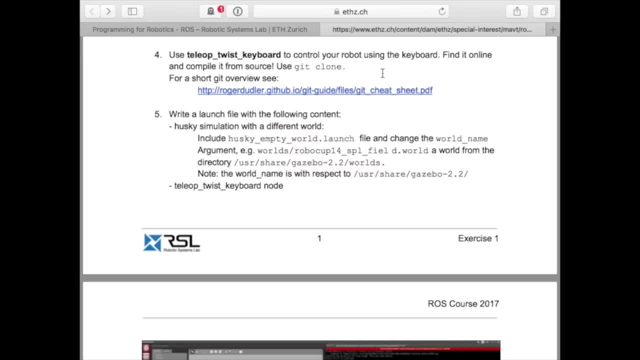 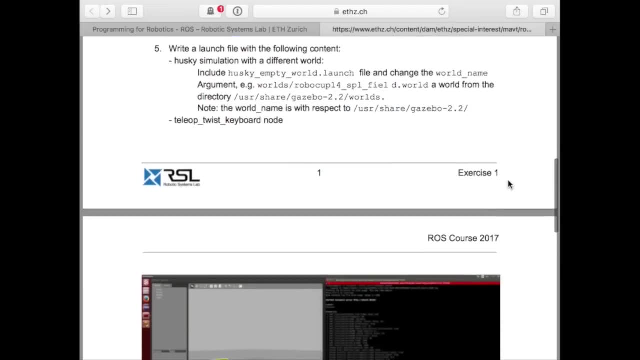 the very basic Git commands that you're gonna need. Then your last task is that you need to write a long launch file, as you've seen before, that XML style file. It has to start Husky in the Gazebo simulation with a different world. So in the directory user-share-gazebo-2.2,. 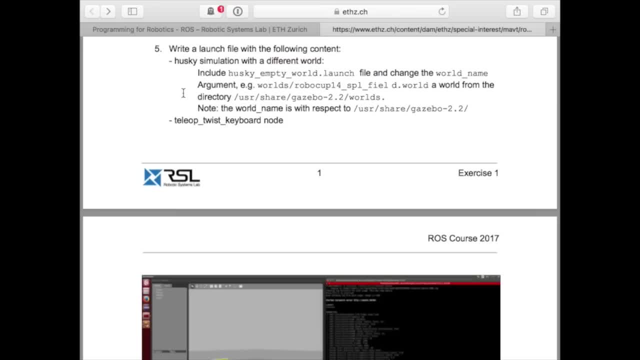 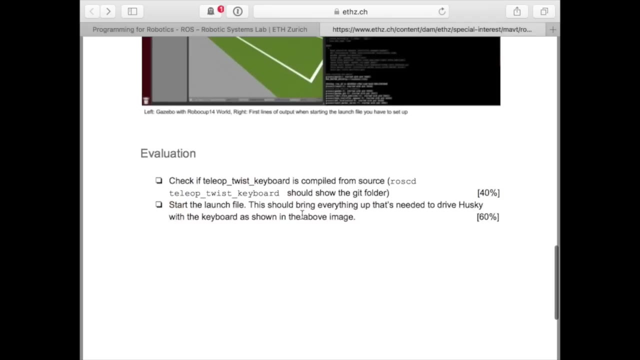 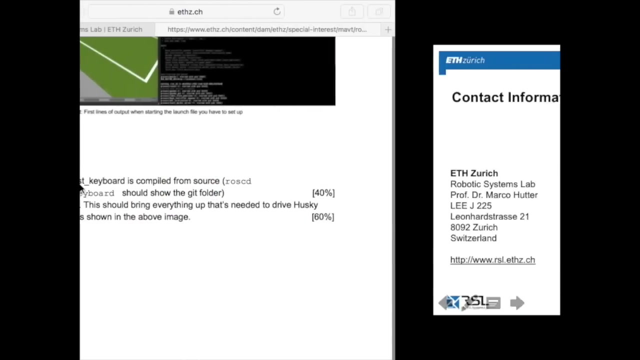 as you see, here there are some worlds stored. You can pick a world that you want, for example the RoboCup world. Then you get the nice RoboCup world that you see in the screenshot here. Now I'll quickly take you through the exercise. So I already prepared that launch file Now. 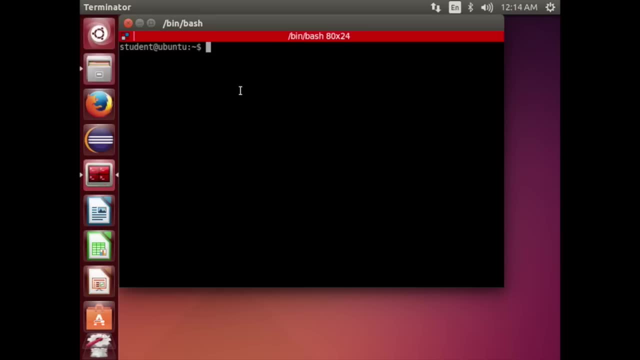 Peter explained to you that you can start a launch file by typing ROS, launch the package name and then the launch file. But you can also go. you can directly start the launch file without the package name, because now you're going to write the launch file and 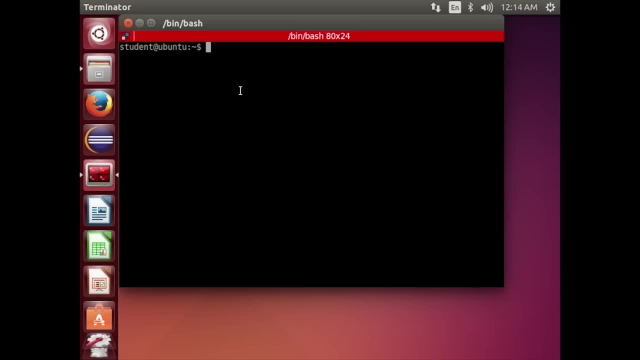 you can change the name of the launch file. But you don't have the package where you can put the launch file right. So you can just create the launch file anywhere in your PC and then type ROS- launch. Then in my case it's an internal repository, So just type. 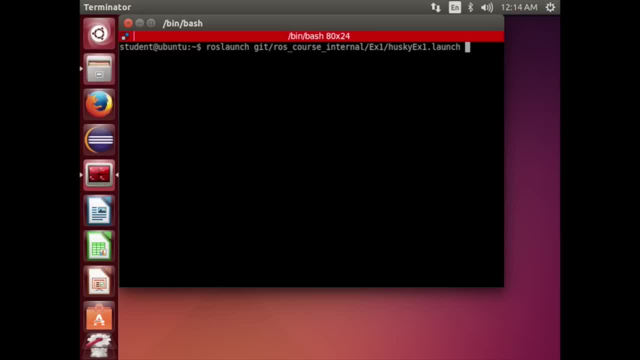 here, ROS, launch, Peter Wiemanen, And then the program gets started. Peter Wiemanen: Yes, Thank you, I'll take it and I'll see you in a minute. Peter Wiemanen: Yes, All right, go ahead. path and the name to the file, and with that you can also start the launch file. 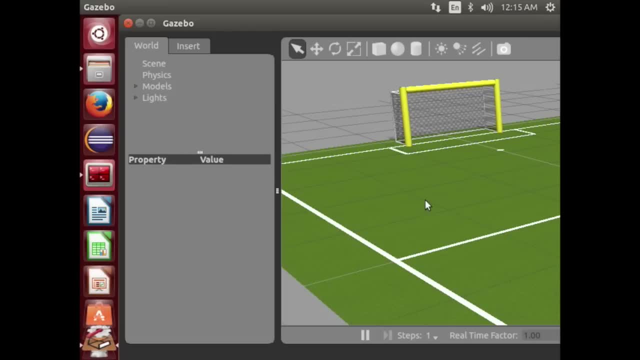 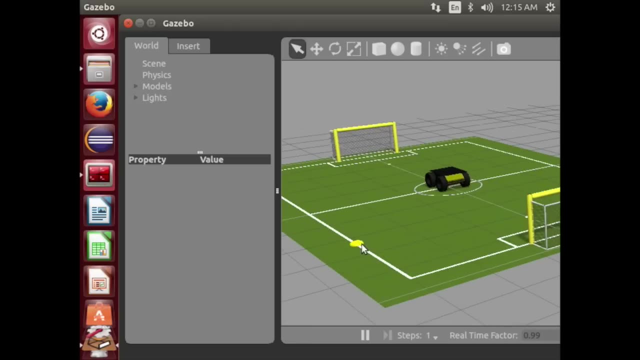 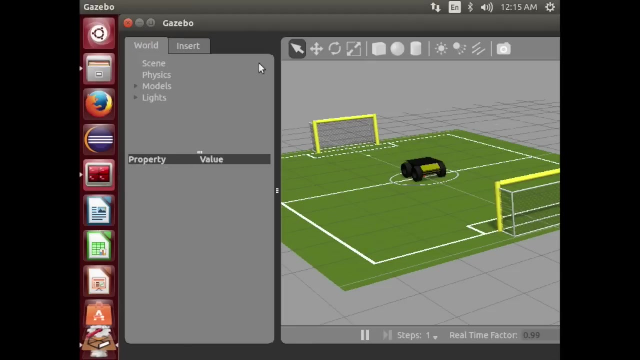 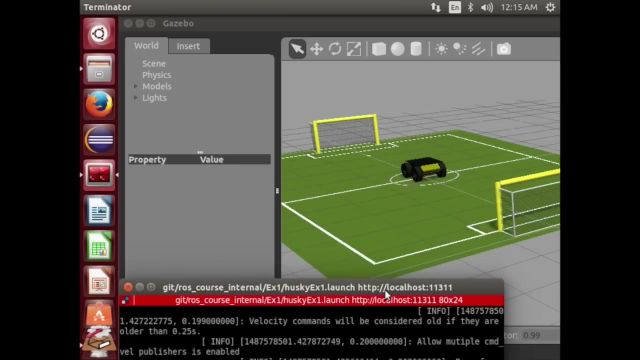 without having a package Now, then it should look better on your PC and the resolution is pretty bad. but now you see that it started the RoboCop world and, as Peter mentioned, you can start stop the simulation and now I can drive around Husky with my keyboard. So for the keyboard to work you have to 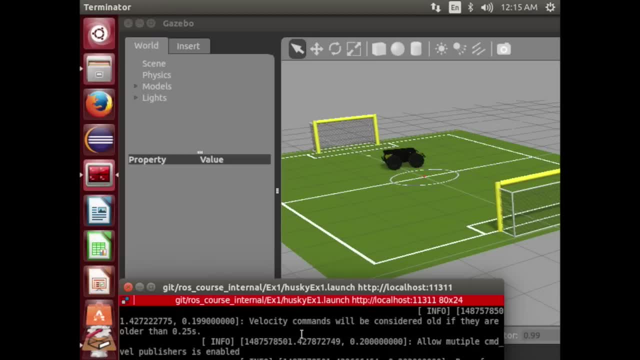 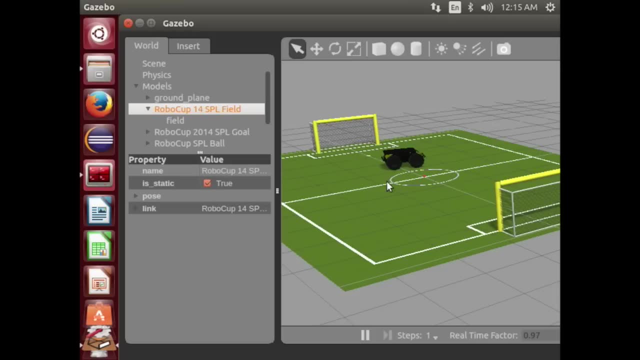 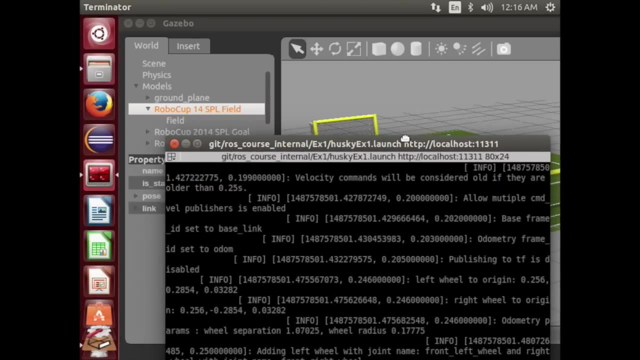 click on the terminal such that it is active the window and not Gazebo. so if I click into Gazebo and then press the keyboard, the keyboard commands go to Gazebo and not the terminal. so that's important. Yeah, so this is the end goal: that you have one launch file. that. 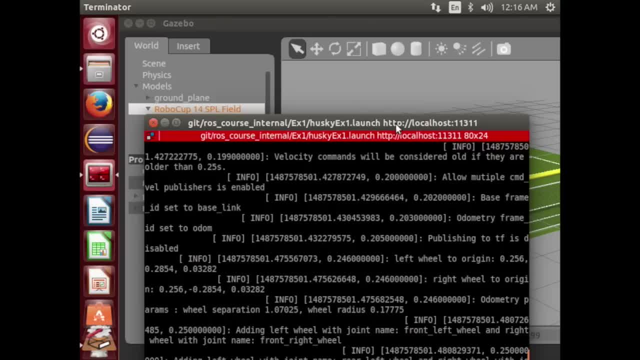 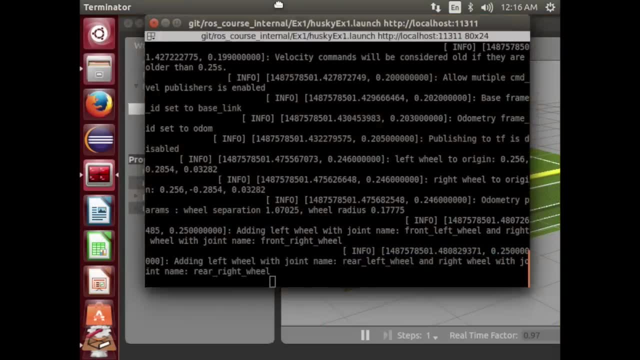 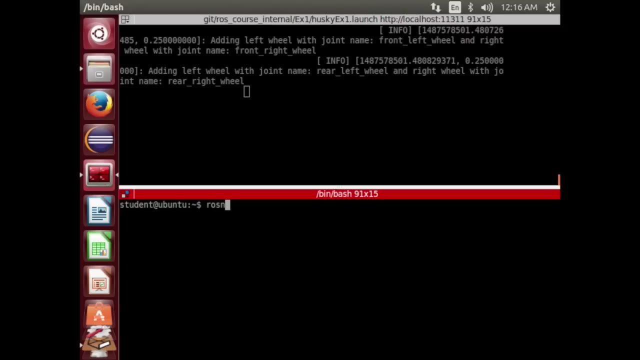 launches Gazebo with a different world, plus your teleop twist keyboard node. Then you can type in all these commands, such as rosnode list. now you see all the nodes running. That's the one that you can have to compile from source so that 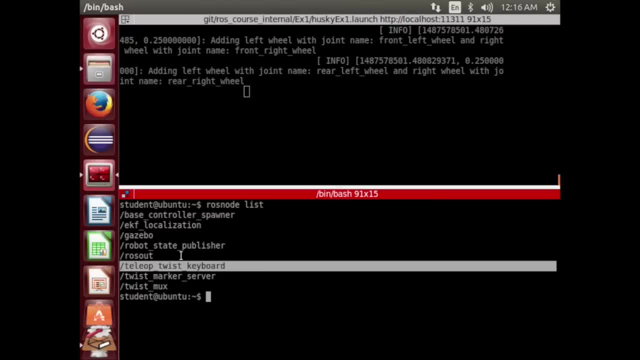 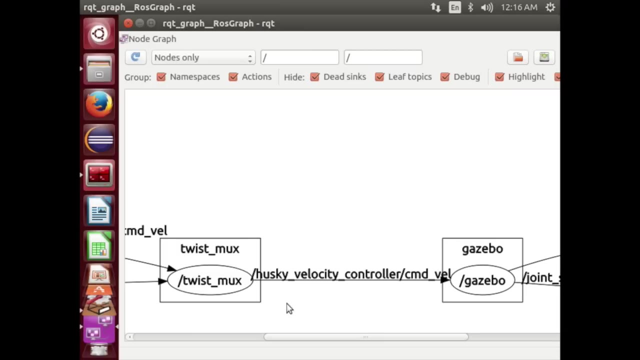 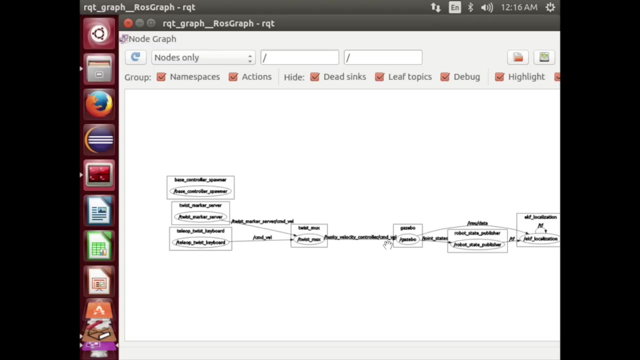 teleop twist keyboard and all the others are started with the Husky launch file. Then there's rqt graph that shows you all the nodes and the topics, how they are connected with each other. You see that here there's a teleop twist keyboard. 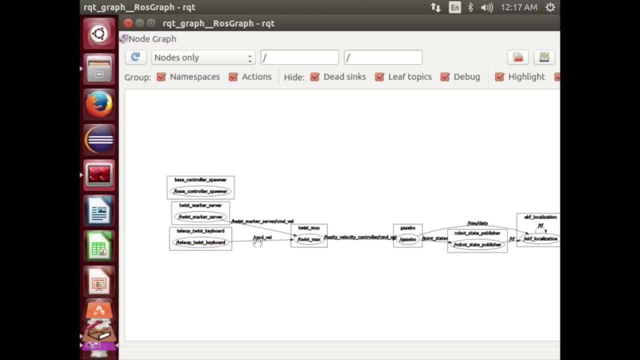 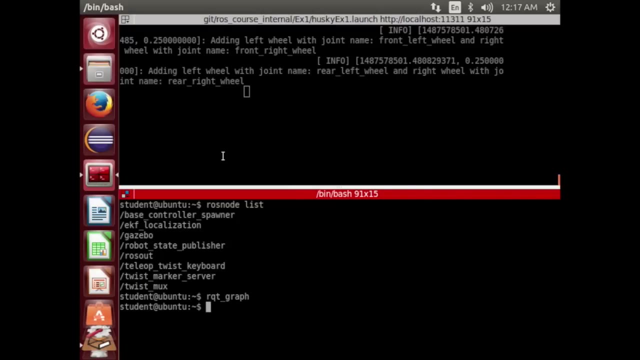 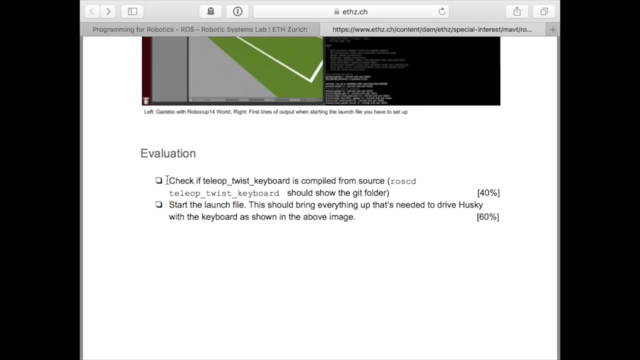 node, the one that I use for the keyboard commands. It sends a command velocity that then goes to Gazebo. so that's how I steer Husky. Now you see the valuation points here. First of all, the teleop twist keyboard node has to be installed from source. and how you see this is when you type roscd. 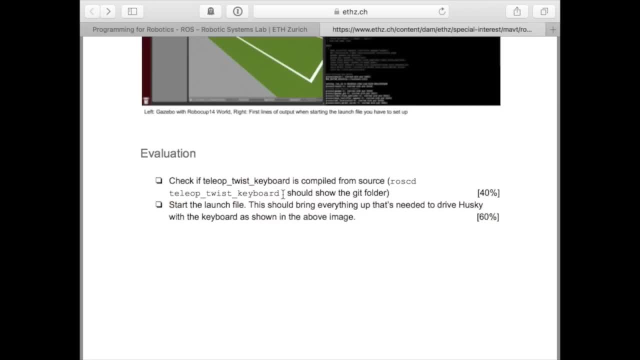 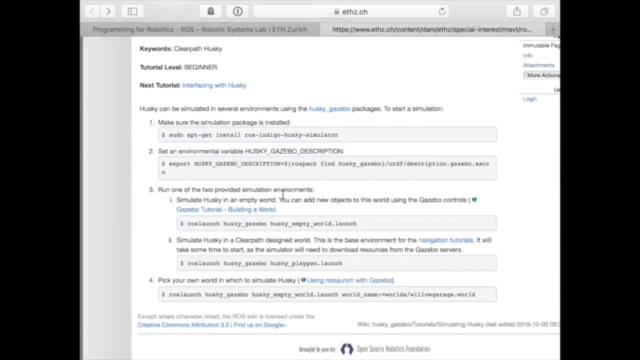 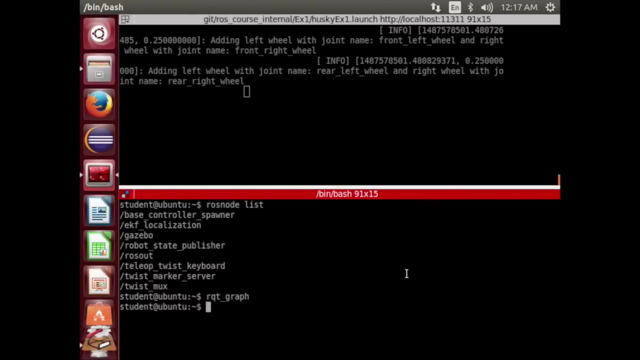 teleop twist keyboard. then it goes into the folder where the source file is stored. and if you, if you would have installed it with the PPA, then this doesn't go into your workspace, it goes somewhere into your system. So I can show this here quickly: roscd teleop twist keyboard. I haven't compiled it from. 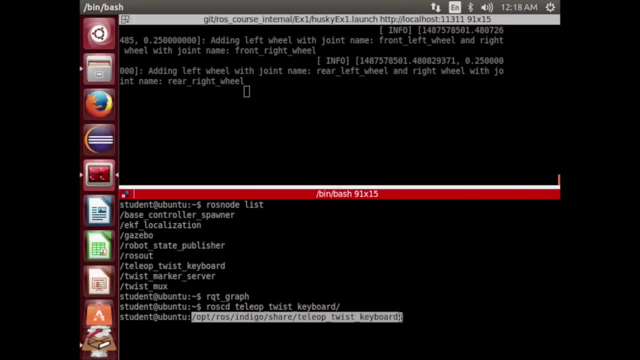 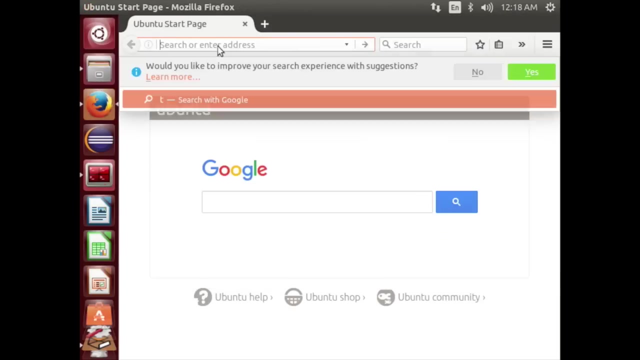 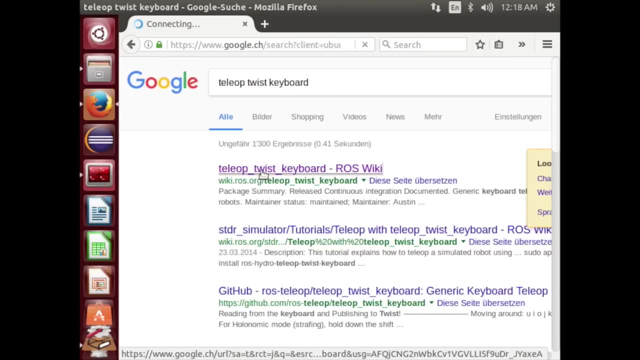 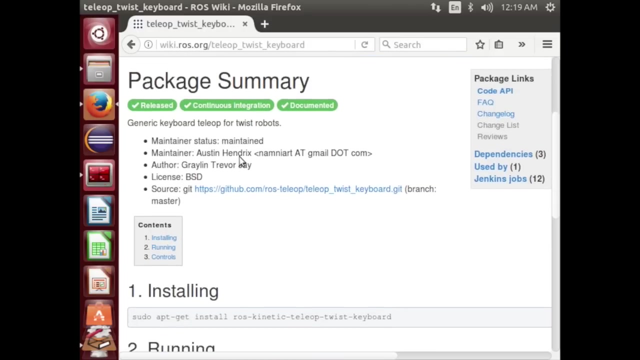 source. so now you see here that there's the system path of roscd indigo share, but in your case there has to be be your username, then catkin workspace source. then you did it correctly, okay, So this is now the ROS homepage. There's there's a wiki page about pretty. 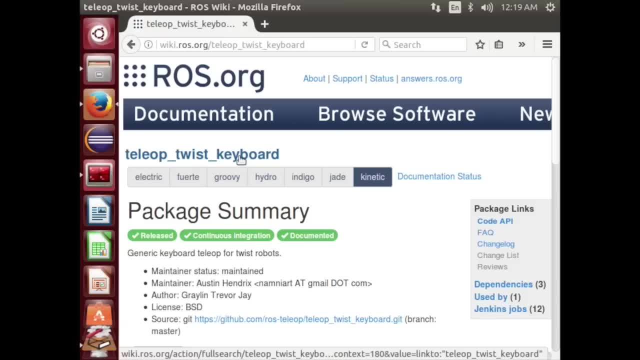 much everything that that's been developed for ROS. Important is that you on top here you have the different buttons for the different versions of ROS. Now we use ROS- indigo and not RoS, So we switch there to indigo, and then there's some information here about how. 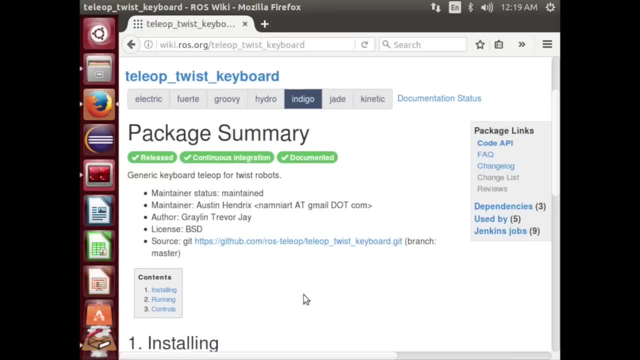 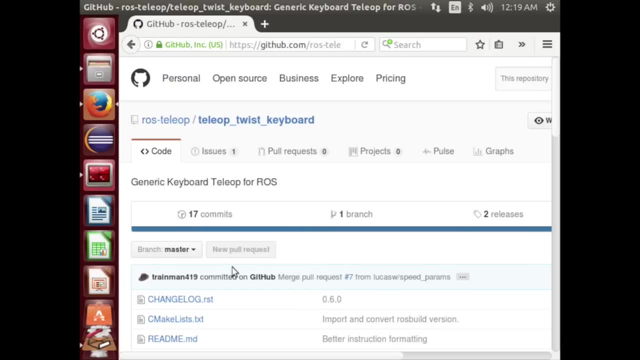 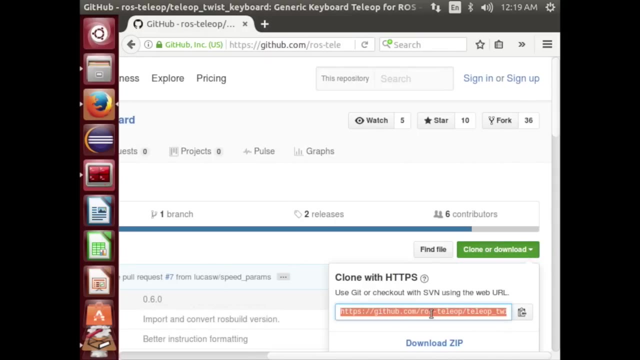 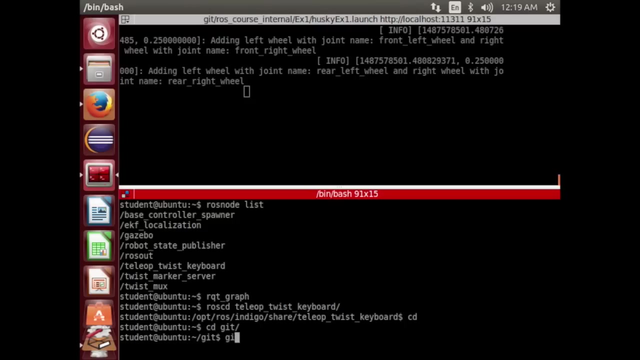 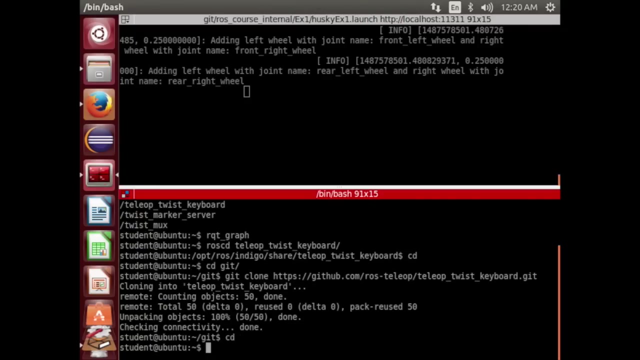 to use it, how to install it and run it. but we want to install it from source or compile it from source. So we go here to the git folder and that's the exact same that you've seen before. You can clone it here. So git clone and then that part. Now I go into the catkin workspace. source. 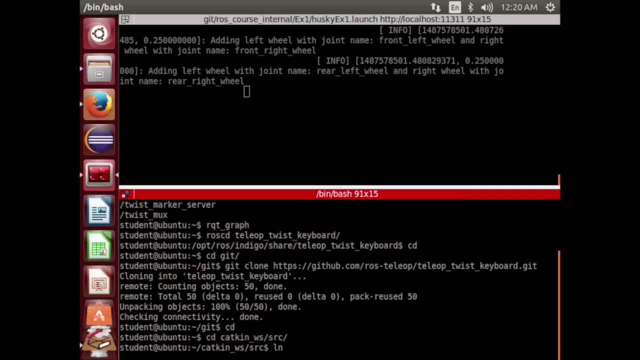 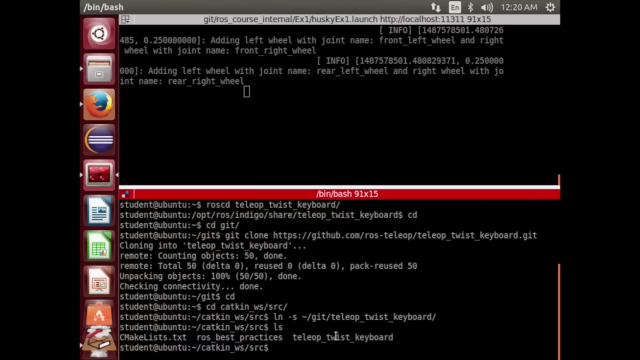 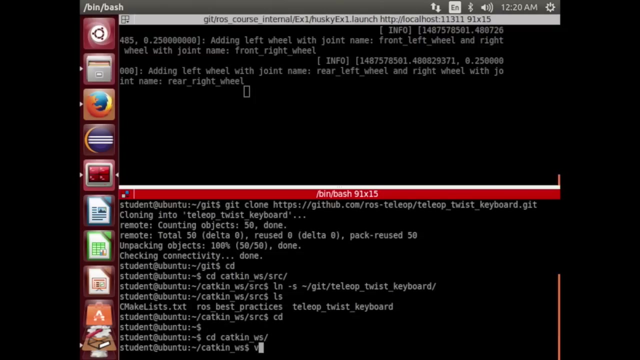 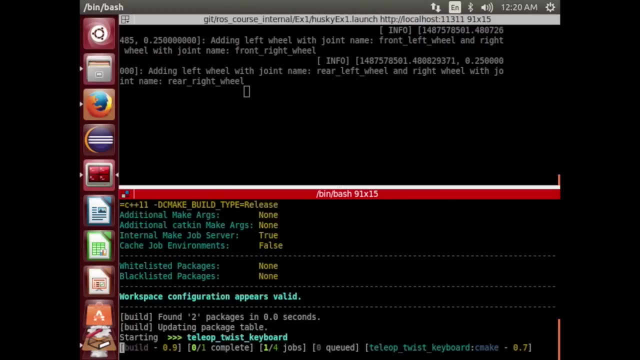 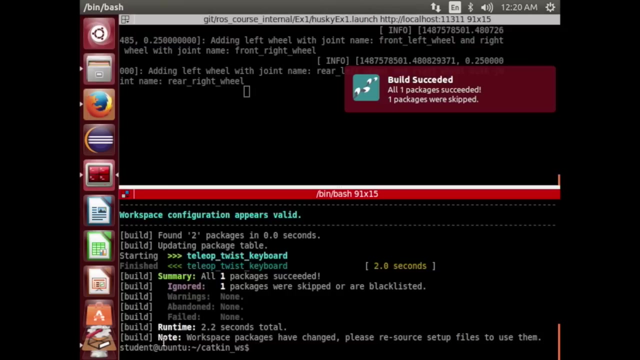 create um, create–, oh-, create- SIM link. Now. you see here that it created that SIM link. Now I go back into the catkin, catkin workspace and build it- catkin, build. Now. important: after you first build a package there's always the note at the bottom that says your workspace packages have been changed.